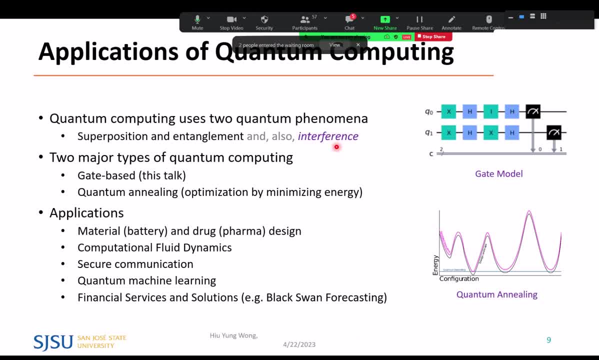 most of the time we cannot get the answer that we want. You will see that later. There are two types of major quantum computing architecture, or I mean a paradigm. One is the gate base that we were taught in this talk. It's just like the gate circuit. 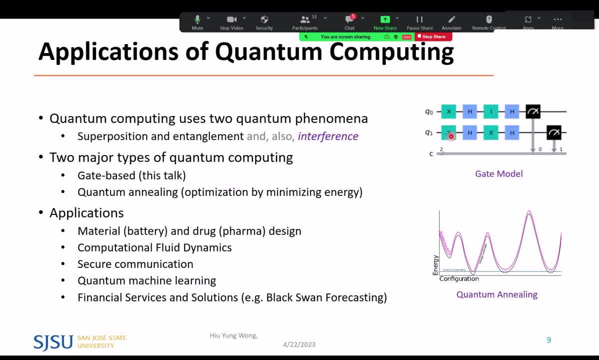 We have a classical logic, but not exactly the same. However, we can think in this way for now. right, You have a state and you keep processing by using different gates. Another is quantum annealing. This is basically like to solve some optimization problem. You 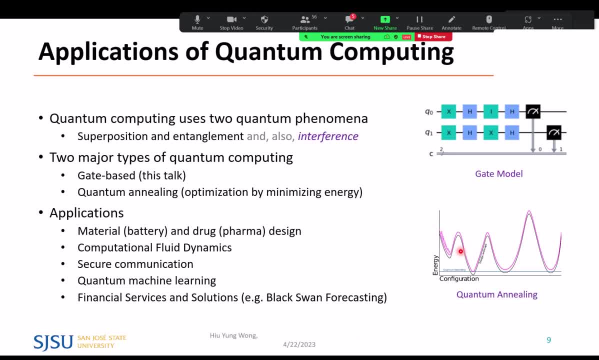 form an energy landscape by using the quantum hardware or qubits, and hopefully you can find the minimum energy quickly, much faster than the classical one, because it allows some tunneling in the hyperspace or the configuration space that they have, And this is something, for example, the d-wave has been doing right And we heard about very many. 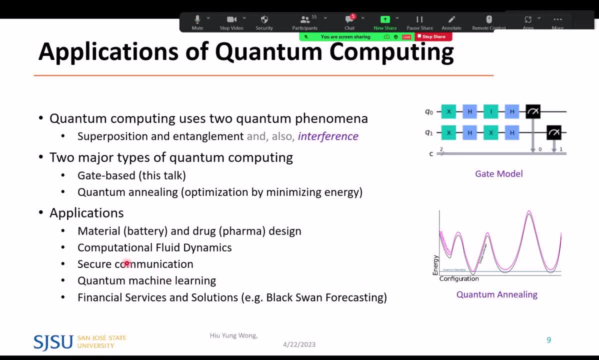 good things about quantum computing. Yes, if it works, it can help you to design battery, design the drug, even do computational dynamics. It provides secure communication. We can use it for quantum machine learning or financial service and predictions, So it's economical. 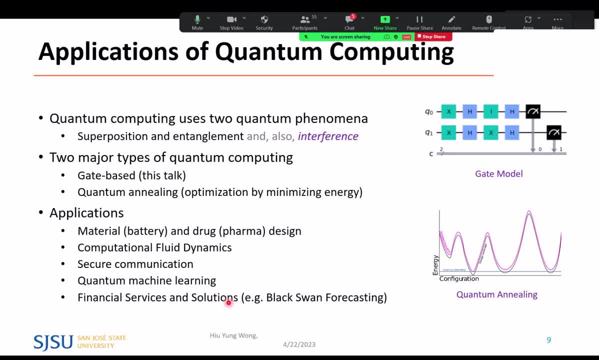 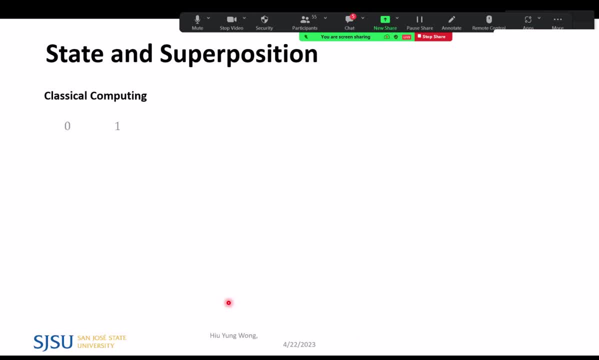 but it's going to have a very big impact in the future. So it's going to have a very big impact and the quantum computing impact is going to be enormous if it is successful. So what is quantum computing? I would say let's look at the classical computing first. 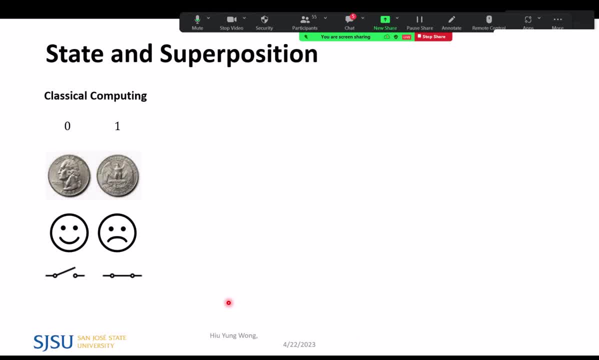 We use zero and one to represent the information. How do we represent zero and one? You can use the coin, head and tail, or even happy and sad, a transistor on and off, right. So we? it represents computing, Yes, but it has something more basic called basis state. It's just like. 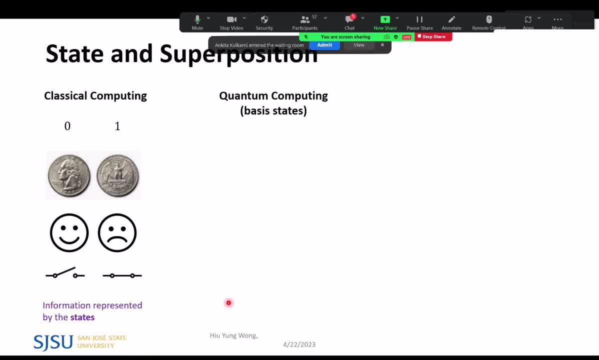 the X hat, Y hat and Z hat on our 3D space. So using the same token, I can represent the basis state, maybe by hat and tail, happy and sad, transistor being on and off, and there's no difference between quantum computing. 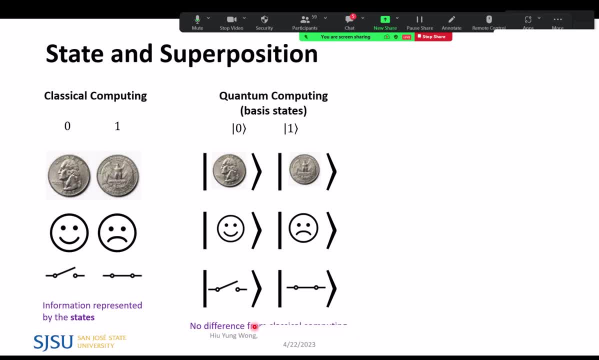 and classical computing if you limit the quantum computer to only operate on its basis state Particularly. here I put a so-called bracket notation. It is nothing but just a notation, So just accept it right. So I represent our state by putting it in this bracket. What's so special about quantum? 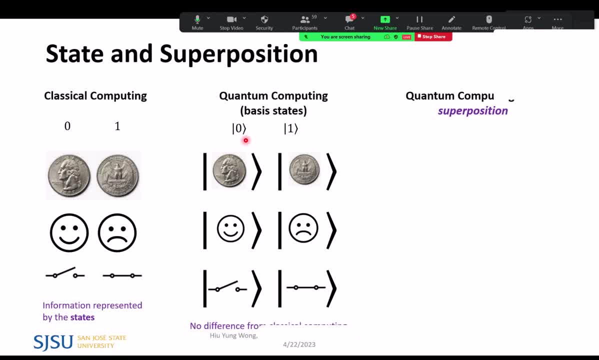 computing is that it also works on superposition. It means that, besides the basis state, I can also have a state which is a linear combination of the basis state. For example, a state sine can be a linear combination of 0 and 1, where 0 and 1 are just the basis state. 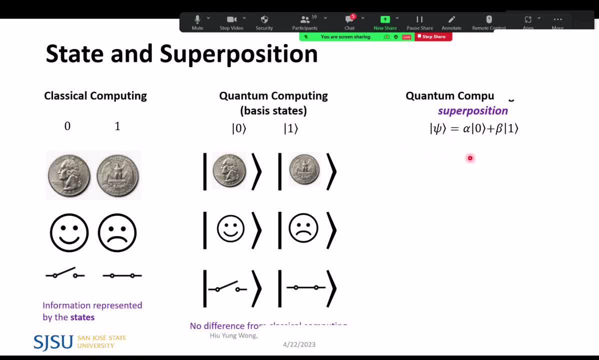 And to describe this state, for this so-called 1 qubit, I need two complex numbers: alpha and beta. Some people would like to make an analogy like this: The superposition is just like a coin that is spinning on your table. You still 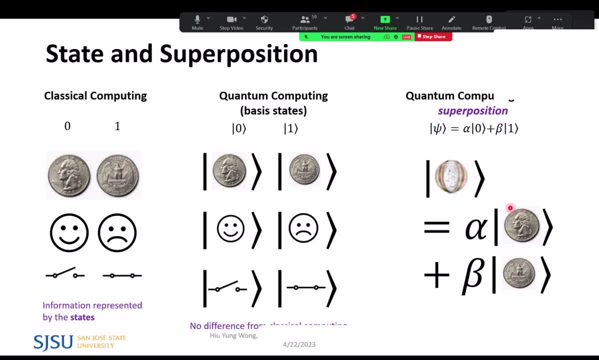 don't know whether it's hat and tail And it's a superposition of hat and tail. Of course, this is just an analogy. You cannot build a quantum computing by using some spinning coins, right? So what's so important is this: On the left: 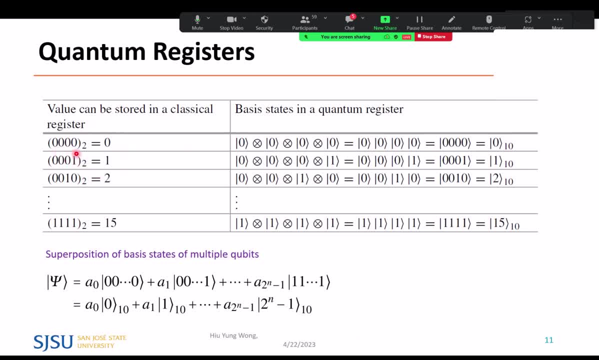 I'm showing you that in a classical register, let's say in this example, I have 4 bits. These 4 bits can represent 16 possible states, And these are just the basis states in a quantum computer. So I can, if I have 4 qubits, I can represent. 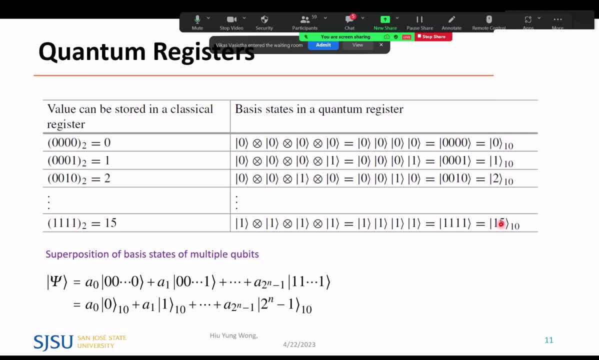 16 basis states, So nothing special. But if I have 4 qubits I can represent 16 basis states, So nothing special. But if I have 4 qubits I can represent 16 basis states, So nothing special. But if I have 4, 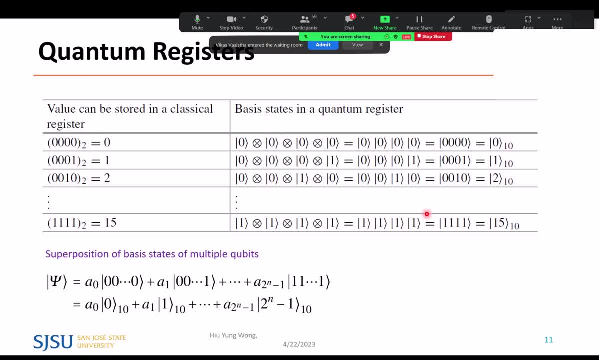 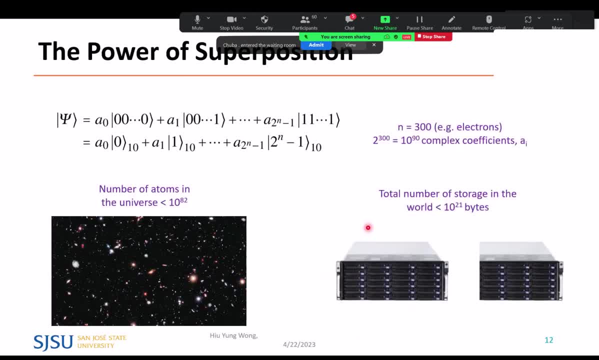 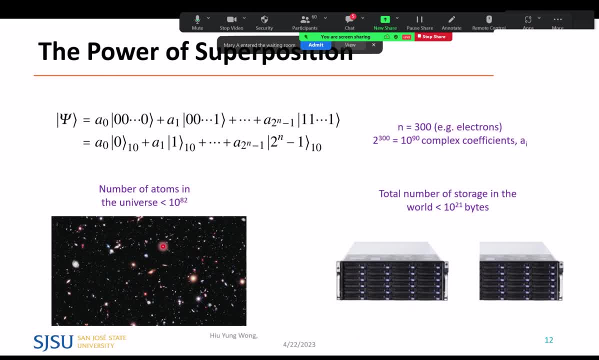 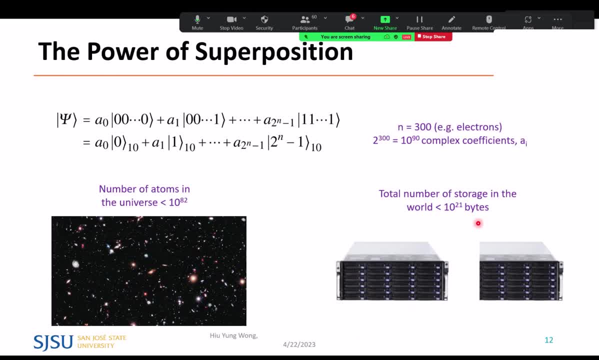 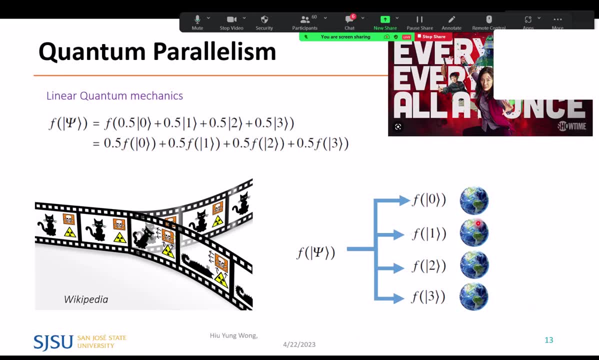 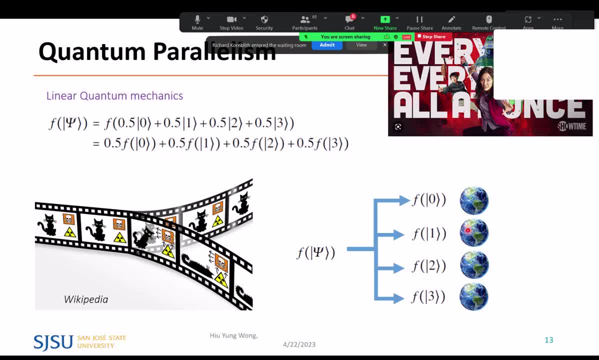 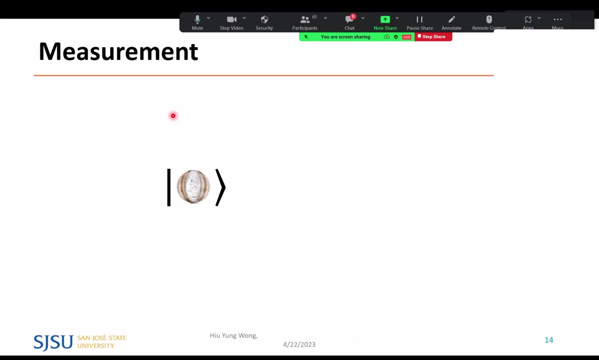 it's just like I have a parallel universe. I have many parallel universe. each of them try to compute the function for me for each basis state. if this work, that will achieve a very important quantum parallelism- okay, so we see is power, then one important thing about quantum computing is how we 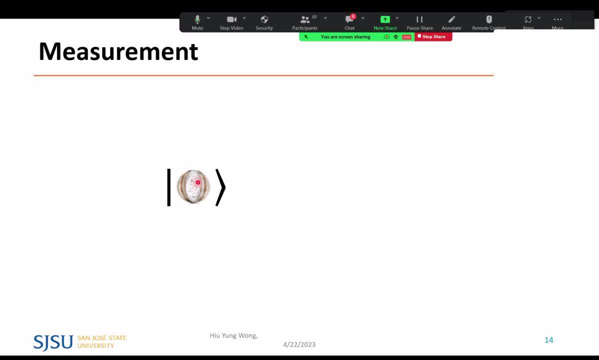 do the measurement? I told you that a superposition state is just like a spinning coin. how will you measure the coin? well, I would just stop it right. what would happen? it may either collapse to head, or it can collapse to tail. that is the same for a quantum superposition state. if it 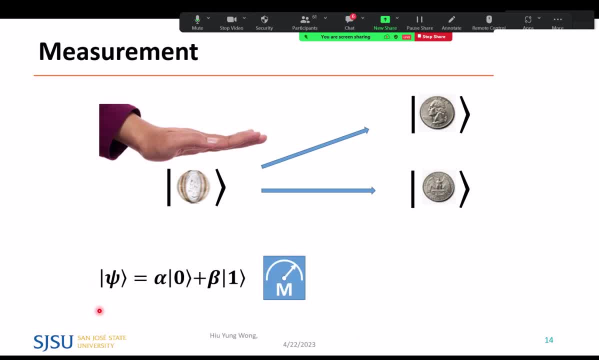 is alpha zero plus beta 1. if i do a measurement, it may collapse to 0 or collapse to 1, so this is completely random. the only thing that's not completely random is that the probability that it will collapse to zero depends on the square of the magnitude of the coefficient. 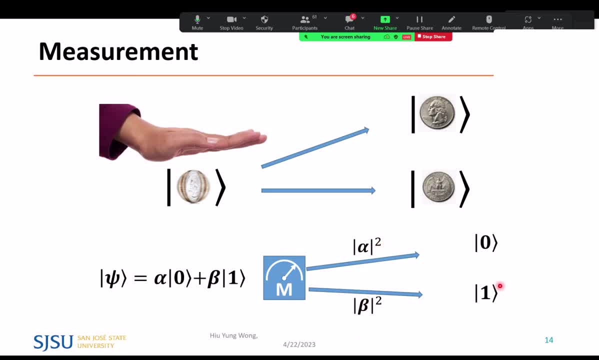 like alpha square in front of for zero and beta square for one. so you see that even i have a lot of information stored in a quantum state. i am not able to get what they are. i need to do a lot of measurement and only to know that, what their magnitudes or their relative magnitudes are. 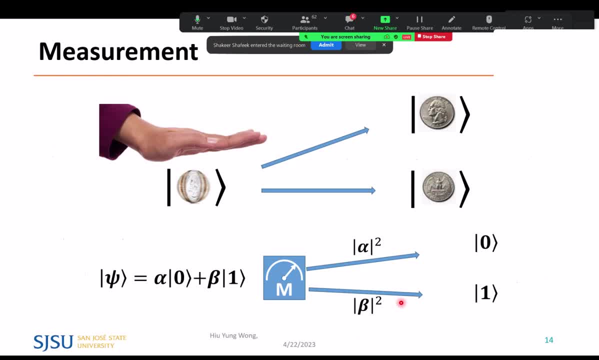 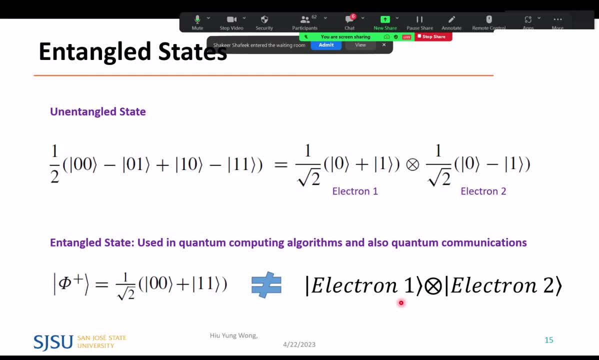 right. so this is one limitation of quantum mechanics, but we will discuss this later. so we talk about superposition. we see it is powerful. we can do quantum parallelism, but it's limited by the measurement. we need to deal with that. another important thing about quantum computing is the entangled state. now, just now i told you that. 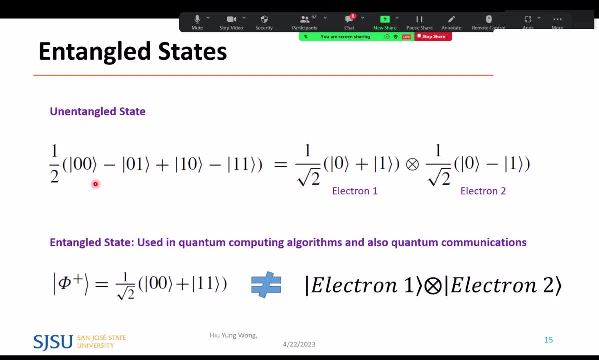 if you have one qubit, you have two basis states: zero and one. if you have two qubit, you can have zero, zero, zero, one, one, zero and one, one. just like the four qubit case, you can have zero all the way to fifteen. now here i'm showing you a two qubit state which form as a superposition of its basis. 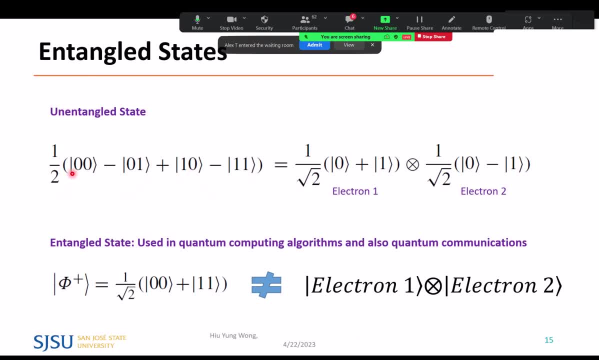 states right. so it's out. it's alpha, beta, gamma or its coefficient. here are half negative, half two qubit state that may come from two electrons. i can so do a some so-called tensor products to factorize it into two states. so basically what it is talking about is that 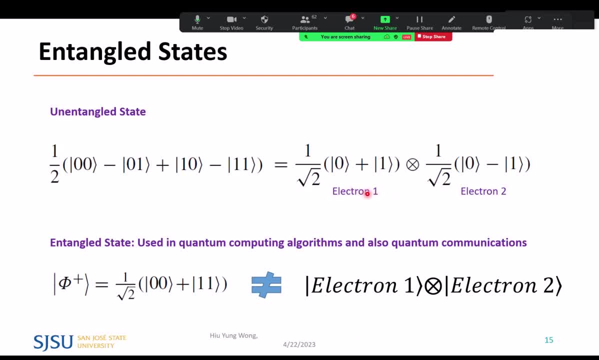 i can describe this whole system by describing the individual system separately and then combine them so they are unentangled. just like before my wife and i marry, i- uh, we are. we can describe ourselves separately and then as a two people, we are not coupling to each other, right. 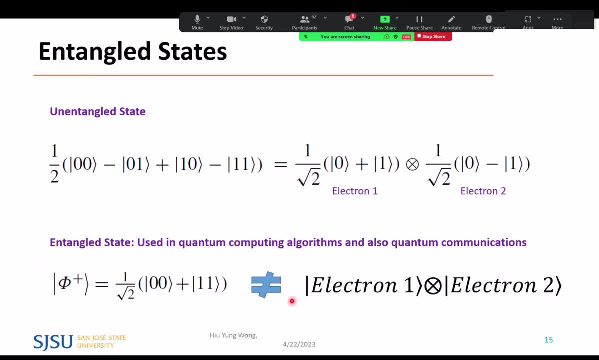 now, if you have a, there are some states you can never factorize it, so that it becomes the tensor product of two systems. in order to describe this system, you cannot describe it from the subsystem. you need to describe this as a whole. this is called entangled state. they are coupled, so this is a very 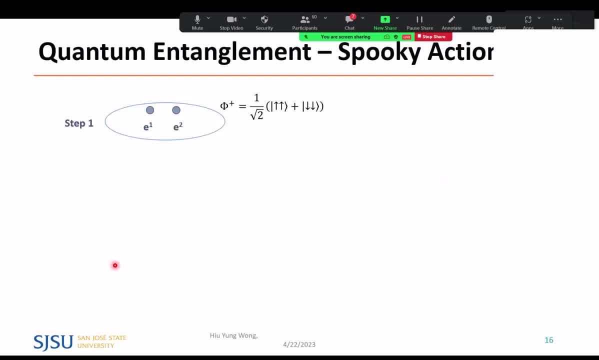 important property in quantum computing- and let's take a look at some- is some special implication. for example, if i create two electrons, i entangle them, i make them in an entangled state. in this particular case, it is spin up, spin up and spin down, spin down. 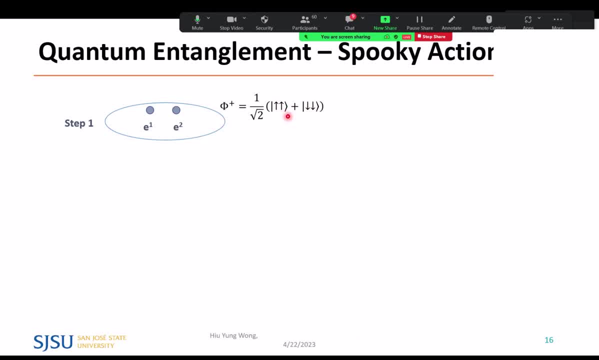 i told you earlier, this is bracket notation. it's nothing but just a notation. inside i can put anything, so this can also be described as zero, zero plus one one, or, in english, up up, spin down down. it's all up to you, right, but we know that it represents the basis state. 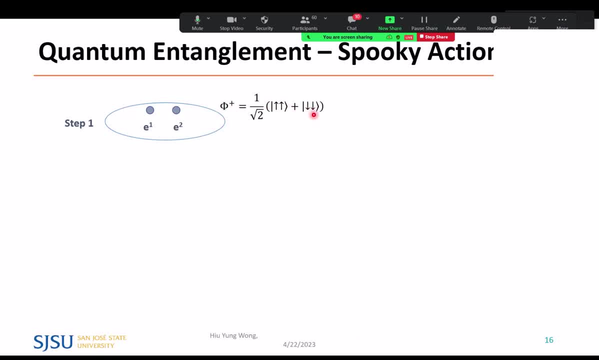 of this whole system which is zero, zero and one one. now i do it very carefully and move one of the electron to 109 years away, so that they are still entangled right, unless they got into- uh, this disrupt, disrupted by some external environment. you can imagine they are still entangled right. 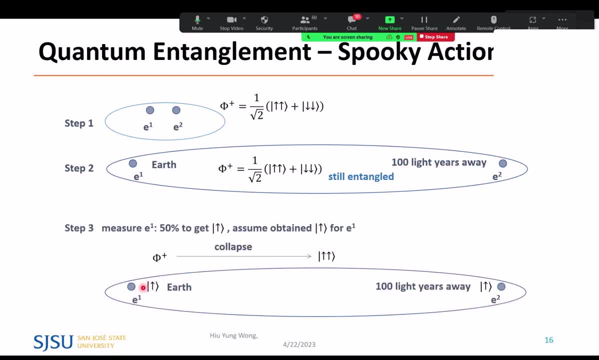 now what happened. if i do a measurement on the electron on earth now based on this combination, you see that it can. it will collapse to either spin up or spin down. that's what we just said. that said earlier, right, any superposition state will collapse to the basis state. so for the uh electron on the earth, you collapse to be up or 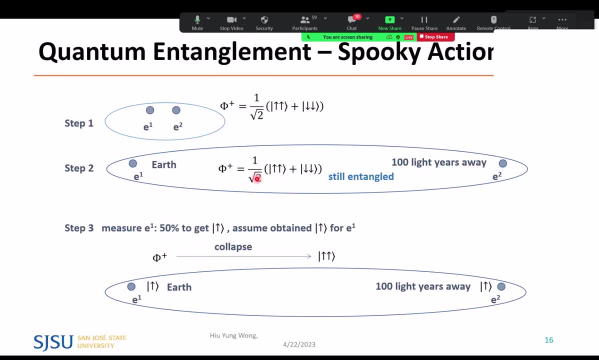 down with 50 because of the coefficient. so let's say i get up now. if i get it collapsed to up. what will happen to this another electron 109 years away? in this whole system when my elect, it only has two basis state that has non-zero coefficient. so the whole system needs to collapse to up up or down down. 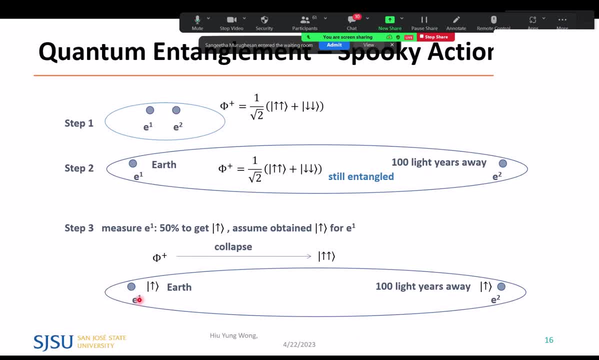 it doesn't have up down. so if my electron on the earth collapsed to up, the electron very far away must collapse to up also. so this becomes something called spooky action for albert einstein. he said how the electron 109 years away know what happened to the electron in earth instantaneously, are they? 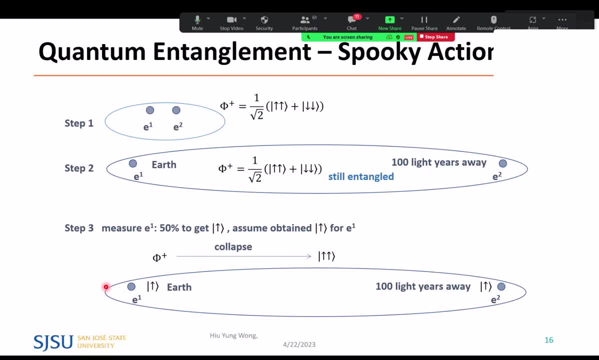 transmitting some information faster than the speed of light. we won't go into the details, it won't right, but this is, uh, just to show you the power or the special of the specialty of this quantum entanglement. but i just want you to remember something called quantum entanglement. 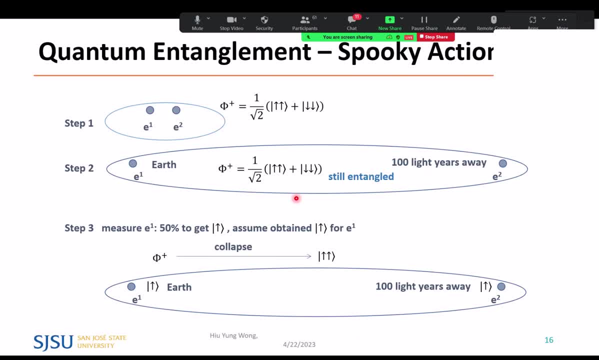 entanglement, that these two uh state are highly important. you could say quite clearly: the quantum entanglement of the earth, at the same time is extremely important to understand. that is why the quantum state is so strong, because, as you mentioned, that the quantum state is very dynamic with and 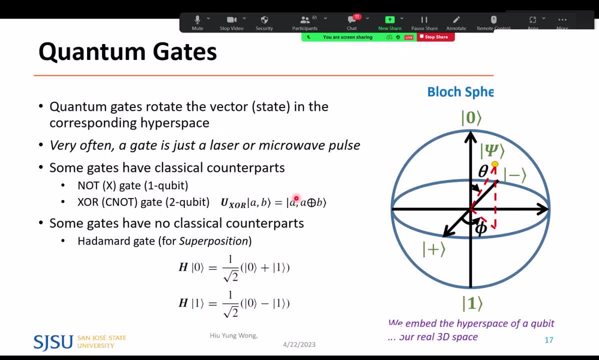 highly correlated. okay, so we look over the basics of the or the most important thing about quantum computing again: superposition and entanglement and measurement, right. so what is the quantum gates then? quantum gates is nothing but just rotates the vector in its hyperspace. again, every quantum qubit or 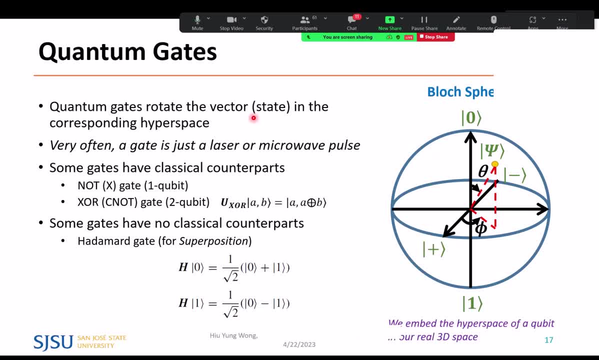 a group of qubit or register. they are just a state right, and this state is a linear combination of the bed state. when you apply a gauge to it, you rotate it in the hyperspace, not in the space we live in, but in a hyperspace mathematical. 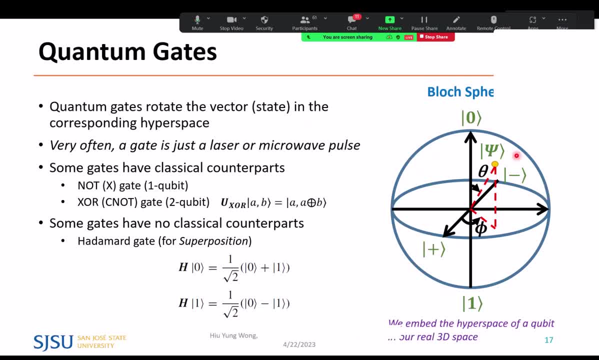 hyperspace and people like to map it to something called broadsphere. when it is one qubit, we won't go into detail, but this Broadway is something sometimes pretty useful but sometimes can be confusing, but anyway, for example, when you have a zero state for this qubit, you apply. 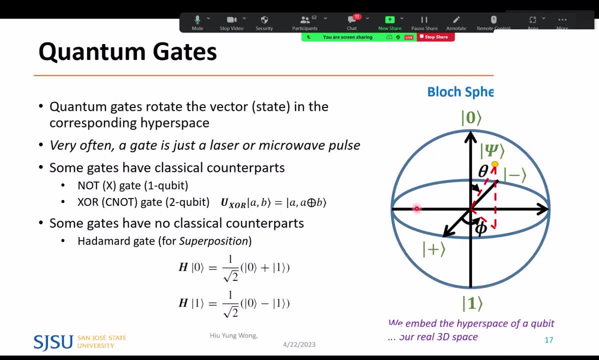 a command in the ПрAy境 fiscal fit and you get a great deal. so this is just a gates. it can rotate to any part on this block sphere and it becomes a new state. How do we rotate it? Very often a gate is just a laser or microwave pulse. It's not. 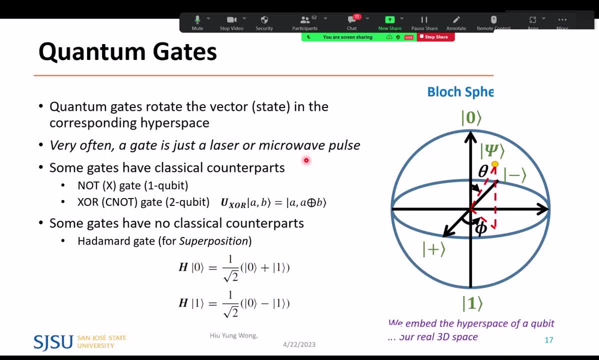 the NOT gate, or a LAN gate we lay out on a semiconductor chip. right, We will discuss more later about that. but remember this: There are different type of gates. Some of them has classical counterpart. For example, the NOT gate, The NOT thing. what it does is just change the basal state from 0 to 1 and 1. 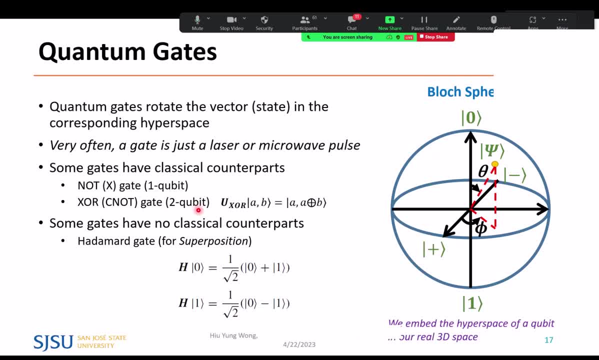 to 0.. It also has two qubit gates, For example a control, NOT gate. So what does it do? It is going to change the second qubit, or what we call the target qubit, from 0 to 1 or 1 to 0. That means apply a NOT gate to it. 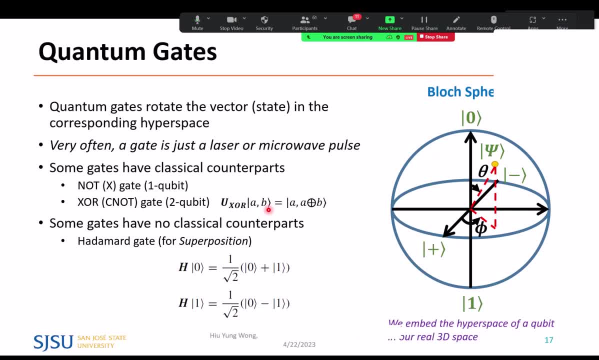 zero, then it's not going to do anything. to the second qubit: okay, but we can build this on a classical computer, so nothing special. as i told you before, quantum computing is the same as classical computing. is you need, if you limit them, to only operate on the basis? 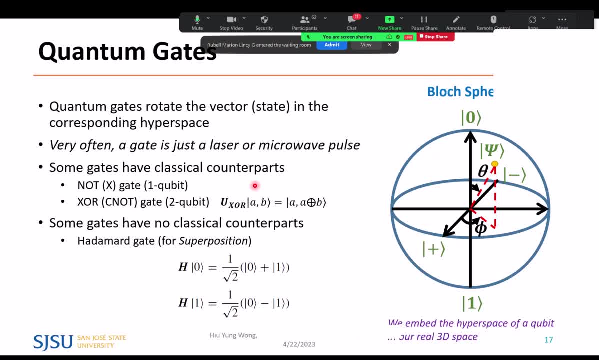 state, if you don't allow they to work on superposition, it's not going to be useful. but you have some gates that has no classical counterparts, for example a hadamard gate. i have a basis. they start from zero. after i apply the hadamard gate, it becomes a superposition of zero and 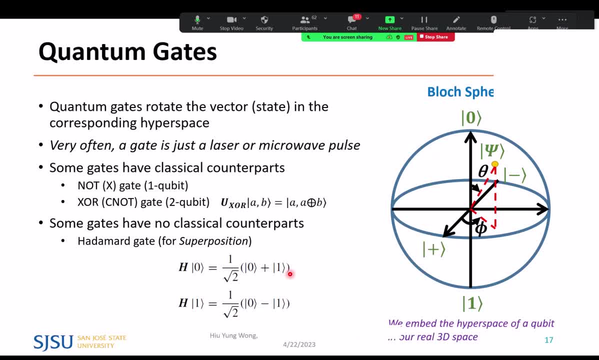 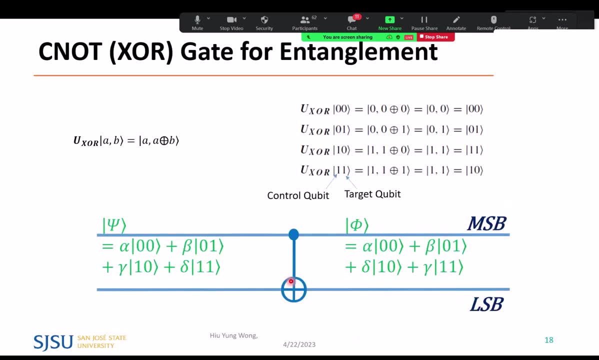 one in classical computer. if you have a register, i ask you what is the content you say? is zero or one, five? if you say zero plus one, we know that this is an error. it must be an error, right? but we can do this in quantum computer. so let's take a look at the quantum computer. so let's take a look at the quantum computer. 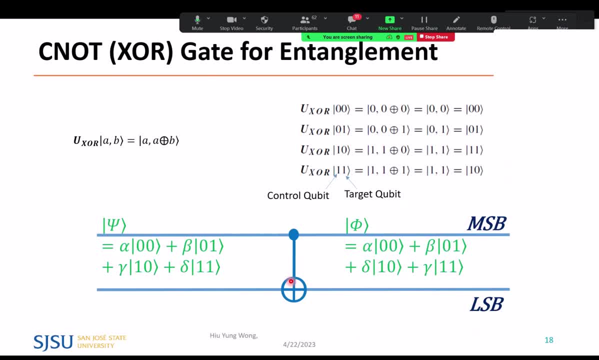 at the control, not gate or exclusive or gate. this is a very important gate to do the entanglement. there are some so-called universal sets of quantum gate, a group of one qubit gate which is easy to implement, and then a few of the entanglement gates and one of the important one is the c. 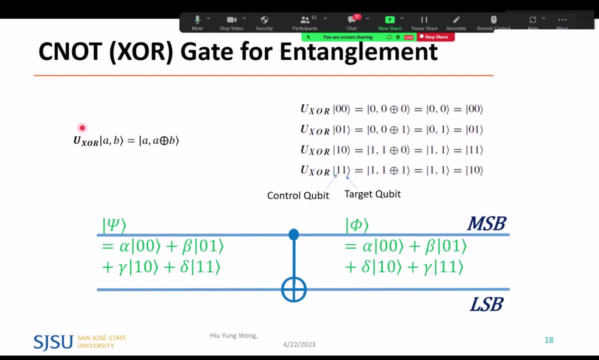 not gate. if you have the c not gate, two qubit gates plus this one qubit gate, you basically can build any algorithm. you can build any algorithm. you can build any algorithm. you can build any algorithm from scratch. so let's take a look what i said earlier. i said that you have two qubits. one of them is control. 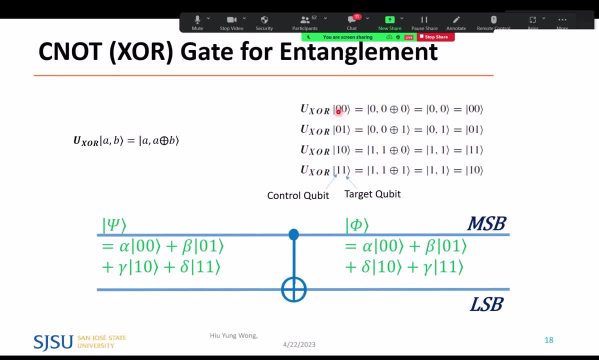 qubit, the second is target qubit. when the control qubit is zero, you do nothing to the second qubit. you see that. so it is still zero, zero, zero, one. but if your control qubit is one, you negate the second qubit. so see, one zero becomes one, one, one one becomes one zero. and here shows: 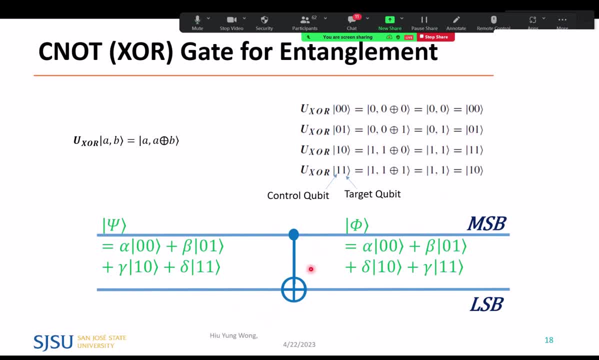 a circuit that we usually draw. we won't go into details, but i want to remind you that in the future, when we read any papers or textbook, make sure that what they mean by the most significant bits and least significant bits in their circuit. in this particular case, i put the most significant. 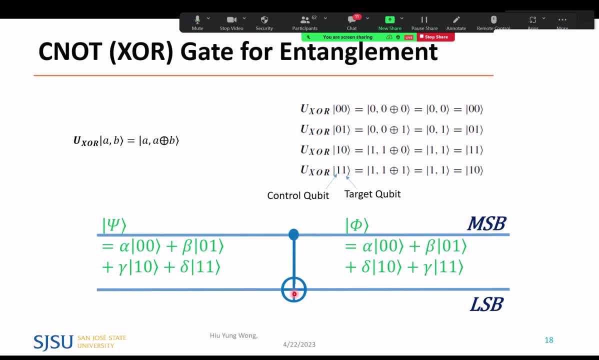 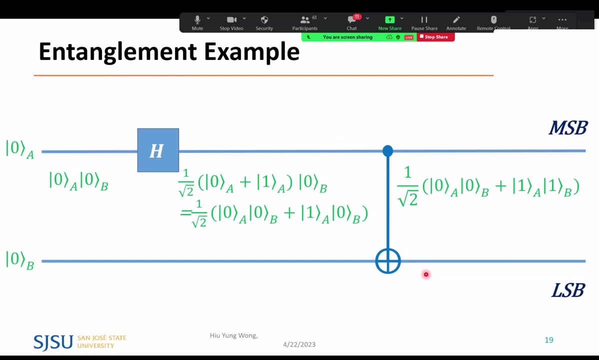 bits on top. so top is the control qubit, the bottom is the target qubit. because of this, its effect on a general two qubit state. right, because i have four basis states right and four coefficients. right is to swap the coefficient of these two basis state. okay, let's take an. 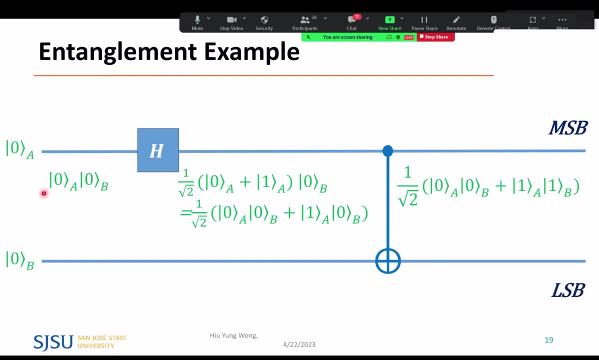 example. look at an example how it does the entanglement. i can start with the ground state, so i have zero, zero. i go for a hardware gate. remember i just told you how domestically is the One Ph likely to increase the speed. so, remember, i use the one phase method. 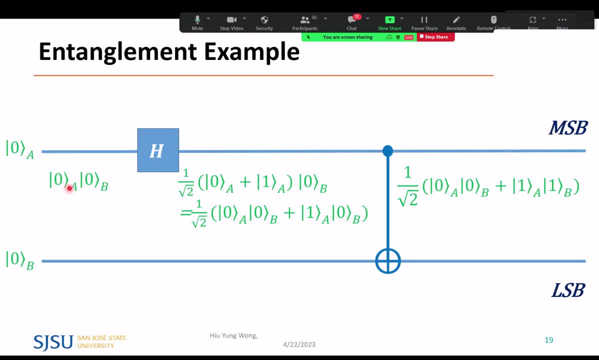 one that can create superposition, so zero. and i only apply to qubit a, the most significant bit right. so b doesn't change, but the a becomes a superposition of it. and then, just like what we do, the in uh elementary school do this distribution law. this is called tensor product. we don't. 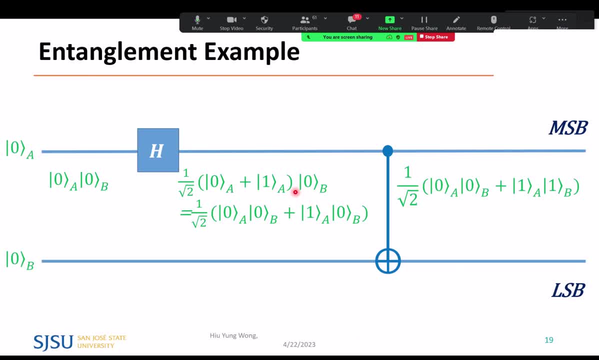 go into the detail, but they have this: they share the same math. then you get zero, zero and one zero. see the superposition of two basis states of this whole system. right, remember what is? the basis state of this whole system is two qubits. so you have zero, zero, one one zero and one one in. 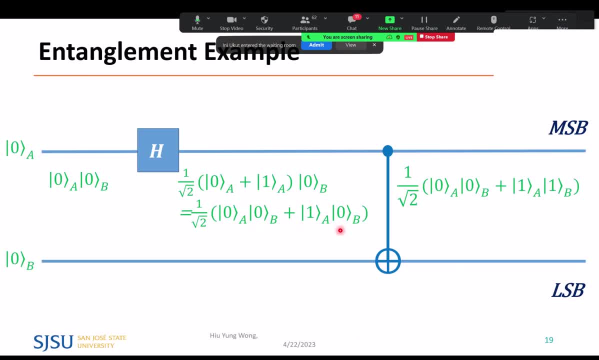 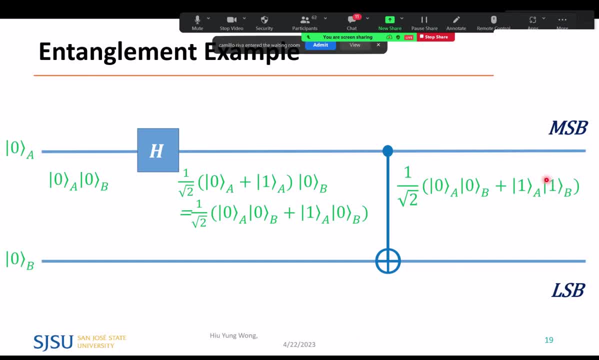 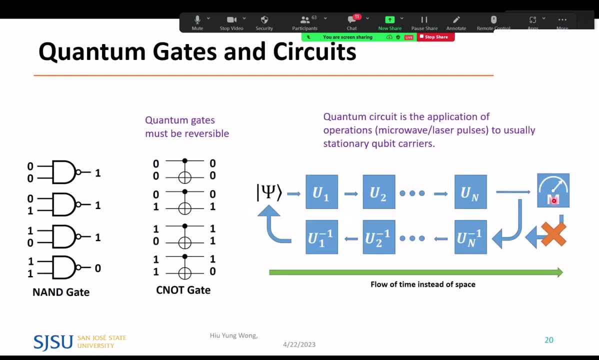 get one one, and this is the entanglement states i showed you earlier in the spooky action slide right, spin up up, spin down, down. so up to here i show you the basics of some qubit and the entanglement gate. and now let's go up to a higher level to understand what quantum gates and circuits 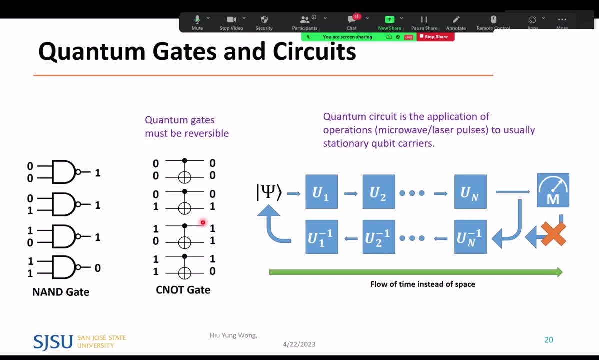 are about. one important property is that quantum gates are reversible. for example, in the classical computing, i give you the gate type and also the output. you don't know what the input is, because zero, zero, zero, one and one, one, zero. four and nine gates, but all give me one one as the 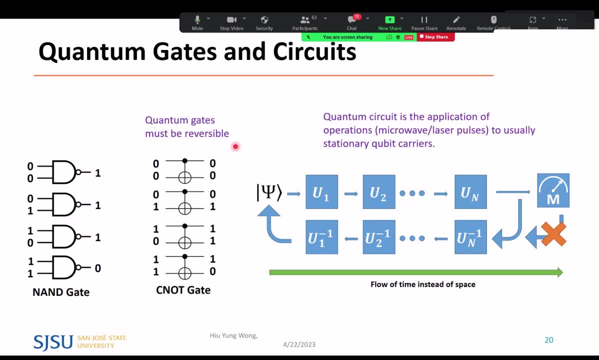 output. so it's not reversible. but quantum gates must be reversible, as you can see here, and that is just because of the physics of quantum mechanics. i told you earlier was a quantum gate. it is just a laser pulse, a microwave power. you apply to a qubit, you change its state. so this is follow the schrödinger equation, so you rotate it in the 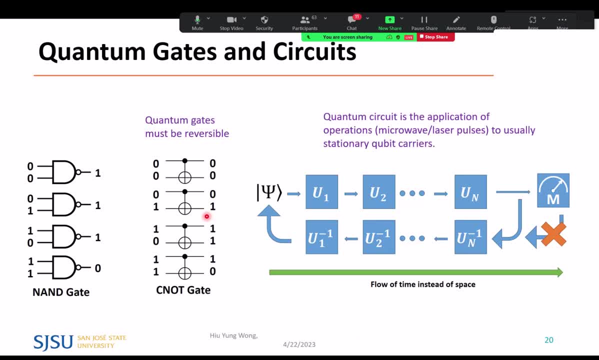 hyperspace. so you can rotate in one diamond direction, you should be able to reverse it in another direction. so here shows usually what we see, a layout of a quantum circuit. and now i want to tell you what is different from the quantum gate and what is different from the quantum gate. 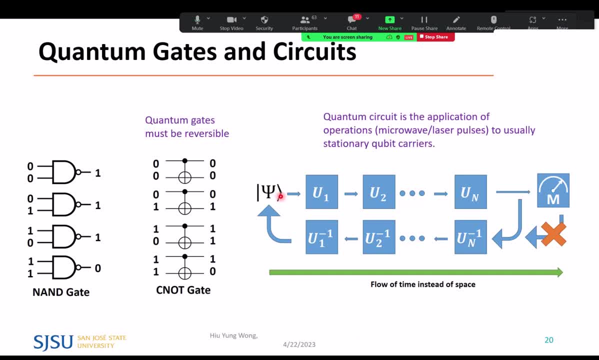 we apply a gate, it means we apply a microwave pulse. it doesn't go through a gate, neither land gate nor gate on our ic layout. we apply a pulse to it, it rotates state. apply another gate means another pulse, rotate it stays again. we apply n pulse and then do measurement. in this process they 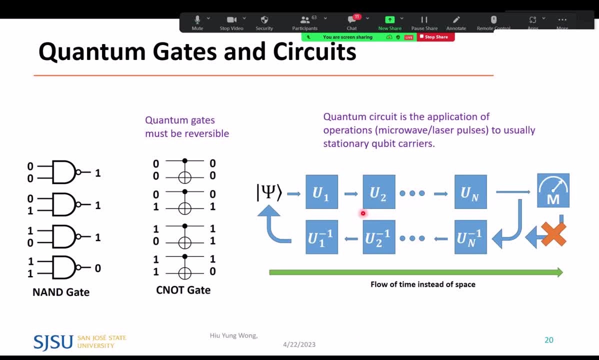 are reversible, as i said. right, you apply a pulse to rotate to that direction. i can re apply another pulse to rotate it to another direction in their hyperspace, not in our 3d space, and but after we do the measurement. we cannot go back now. do you see that? this is the flow of time, not a space. so in 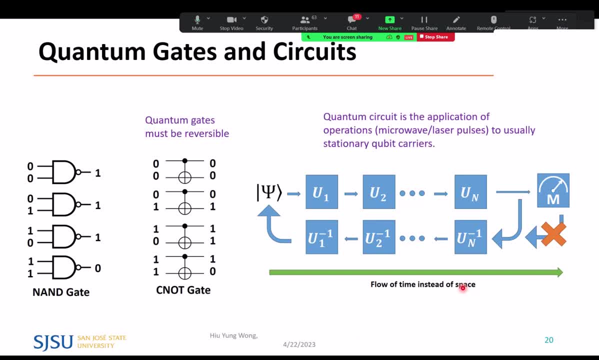 some algorithm you see in the future. they say that you need to apply one billion of gate. you will get very nervous if you are ic layout designer. well, i need to apply one billion gate. that is impossible or difficult in ic chip right in a train, but here just means that you keep applying the same. 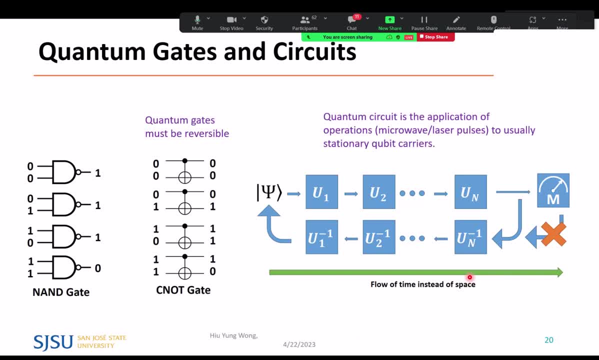 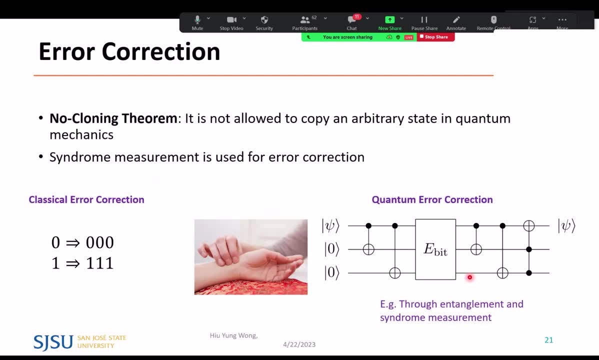 microwave i mean different microwave pulse: 100 times, 1 million times or 1 billion times. okay, the last topic of the part one. what i talk about. what i talk about is about error correction. now, in classical computer usually we will do duplication to avoid, to avoid the error. right? i call my mom. 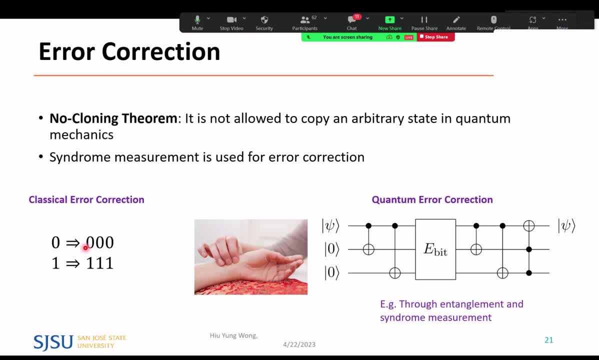 in asia and i say something to her she cannot hear. i keep repeating 100 times, at least maybe 50 times. she heard that. then she get that as the answer. but in quantum computing it doesn't work because there's something called no cooling theorem. you cannot copy an arbitrary state. okay, so then what? 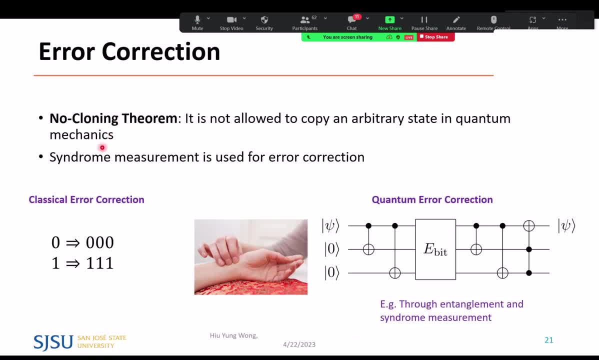 can we do? uh, one of the method is called so-called syndrome measurement. just like i like some medicine or traditional medicine, like they don't really test what you have, they look at the syndrome. right, if i'm coughing, i don't know if i got covid or just regular food. i went to the doctor. one possibility: 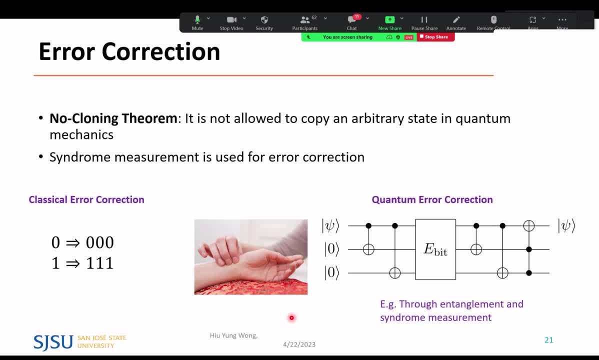 instead of testing my blood or my saliva. maybe the doctor is so experienced. how often does you cough? what's your fever? my heart beat and then maybe the doctor came up with a conclusion: oh, you just have a regular flu. that is what we do in quantum computer, also for error correction. psi is a state that i care. i care. 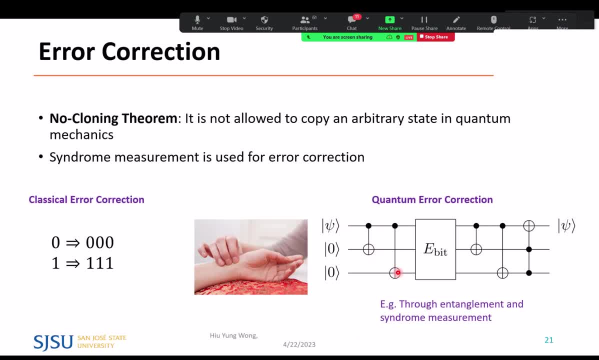 about what i do is apply some synov gate to entanglement to to some auxiliary qubit and then maybe i got some error. this is just a gate to mimic the error. through this i can just measure this gate and then do appropriate operation to side based on my measurement open outcome. so here, not just 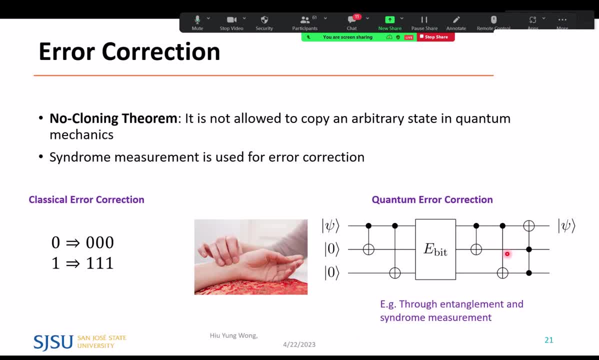 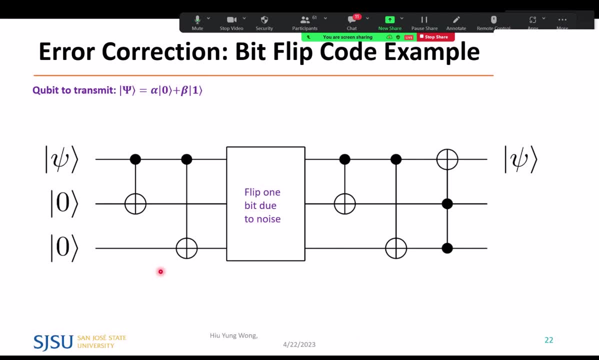 that we have measurement. this circuit is just that you do the automatic correction. let's take look, take a look. and on an example again, i said the side is what i care about. and then i it is in terms of alpha zero plus beta one. i don't know what is alpha. i don't know what is. 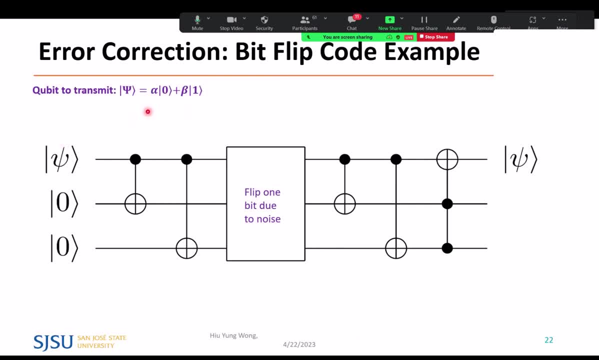 beta. right again, this is b, when you get to the point where maybe it's your middle finger finger, your lower, father's pulls your thumb just so comfortable with the smooth lahmin time, because that gives you one qubit. right, because i have two basis states, zero and one and two coefficient. 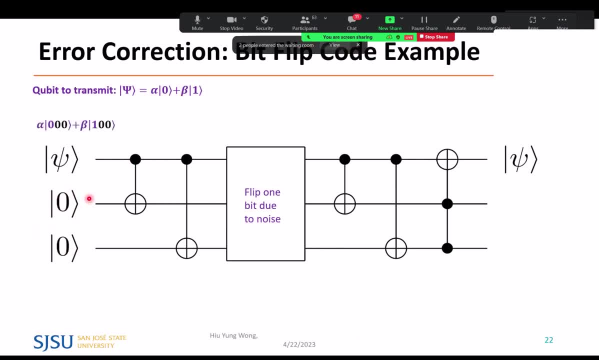 so what i do is combine with this auxiliary qubit, starting with zero. so what is the basis state of this whole system? because these two are zero. so i only have zero, zero, zero and one zero, zero, right, i have three qubits. i have eight. basis state, remember: zero, zero, zero, zero, zero one. 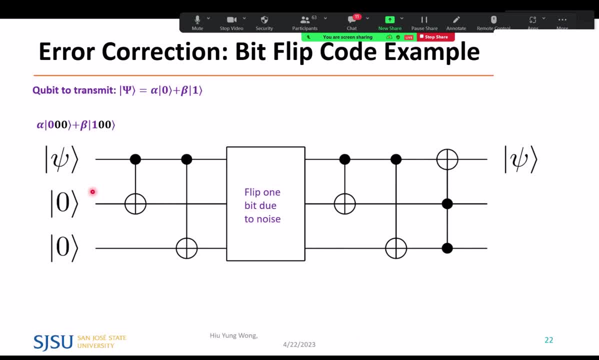 zero, zero, one zero all the way to one one, one right. but because these are zero, so the whole system combined with sine is just zero, zero, zero and one zero, zero. then i go through the first, control not gate, and the second, control, not gate. again, control not gate says that if this is one. 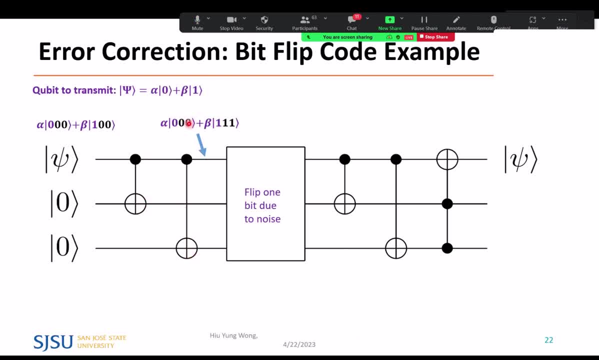 negate it. if this is one, negate it. for the first, first basis state: this is zero, nothing changed. for the second one: this is one right. so i change zero, zero to one one. so you see it's entangled. that's why we say this is a process of entanglement, which is very important. let's say i'm very unlucky. 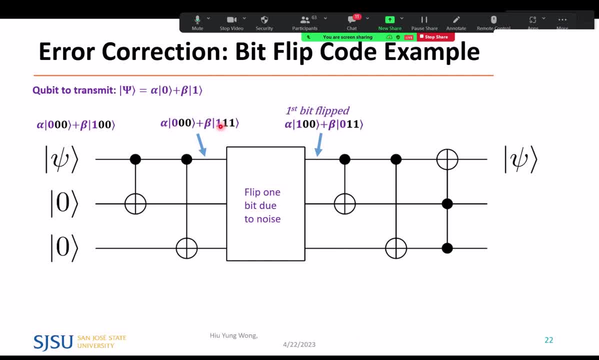 i got the first bit flip. it was one zero, zero. one. now becomes one zero. it's free right. so this circuit will save me why now i have another control, not gate it. say that if this is one, flip it, negate it. if this is one, they get this one. so look at this: this is one right because it got flipped. so 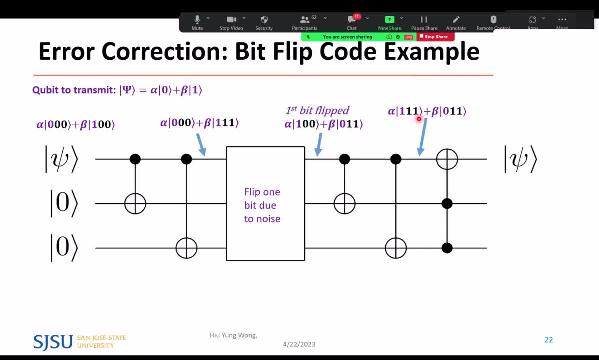 it's going to only get zero and zero. so i got one, one one. the second one is zero. here then i'm not going to do anything because it's the property of control, knot. so i still get zero, one, one right. so with this, then, what happened at the? 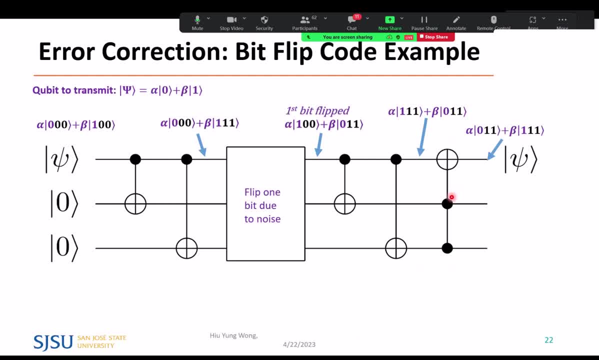 at the end. how do i correct with this circuit? this is in a so-called control control knot we did not discuss. it means that i'm going to negate this bit if both of these are one. now look at this: both of these are one, so i mean here, both are one, so i'm going to. 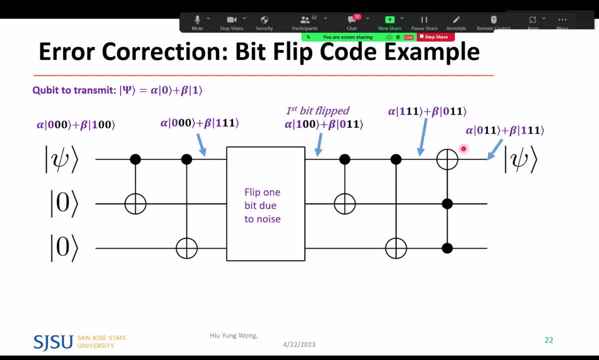 change that to zero, both of one. i change this to one and you see that through this operation i recover psi equal to alpha zero plus beta one, because i don't care of this auxiliary bit. so in quantum computing, where algorithm very often you will see the so-called auxiliary bit. 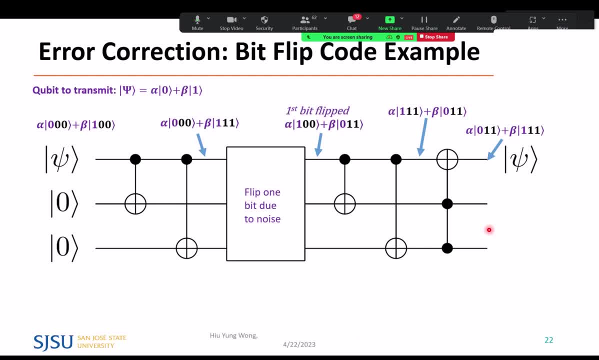 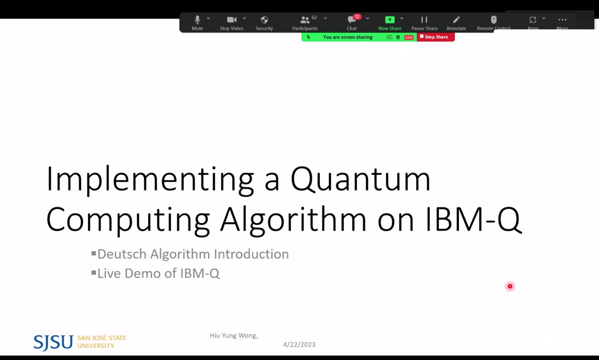 that or ancillary bit. they're critical for the operation but you discard them at the end. okay, try different type of fit flipping. right, they can also flip their auxiliary bit. you will find that you can correct that. okay, at this moment i would like to just show quickly an algorithm which is called 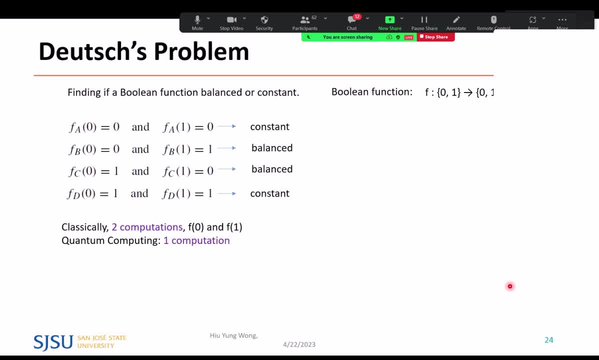 Deutsch algorithm and just so that you have an idea on what what it is about, right, so Deutsch algorithm is a is something that help you to effective fun拉 phil server. right, right, when you take our ic one 10 billion transition or one billion transition, do you meets the timing criteria? this is yes and no question, but to answer this question is super. 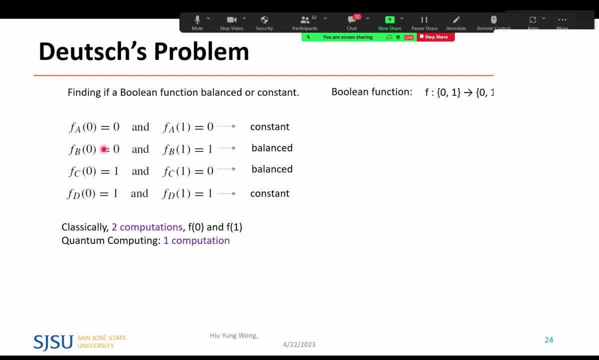 difficult, right? so here is a simple question, well, one of the one of the relying if you answer something. a simple question, very simple, just i mean a simple example. it only takes one bit, zero and one, and output zero and one. i want to ask whether this function is constant or it is balanced constant. 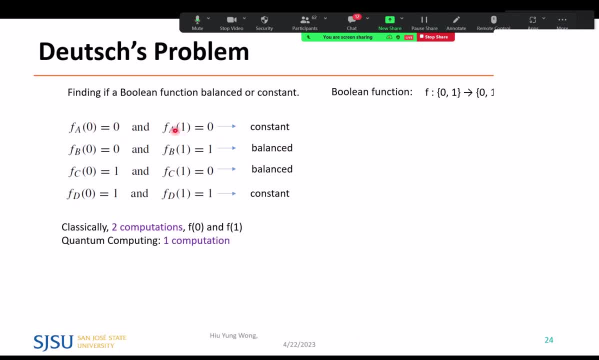 means? means whatever i put in it gives me the same output, for example, constantly zero or constantly one. balance means that whatever i put in it always give me i'm not whatever, but for all the vector i put in it, always it will give me half zero and half one as the output, and that is called balance. 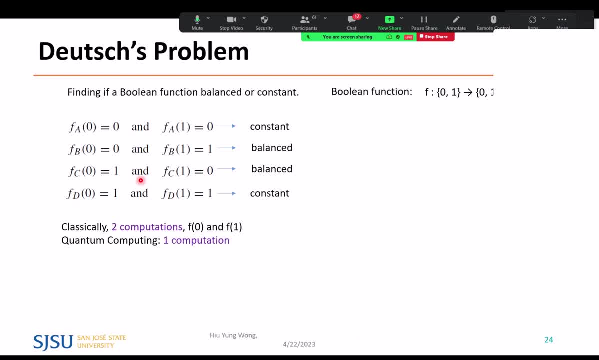 now in classical computing, if you don't know what the function is, what do you need to do? for this simple question, you need at least two computation, right? okay, i have some video for this you can, which is out in the video that i showed you earlier. right, you need at least two computation. but for quantum computing, i only 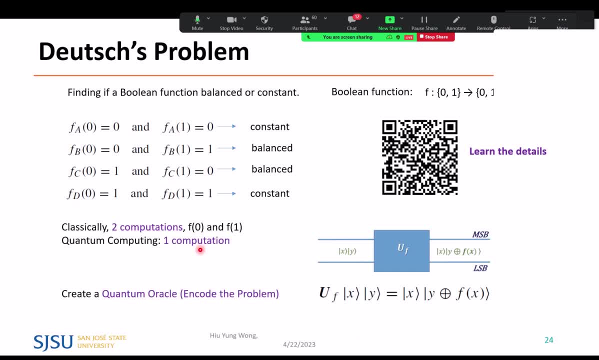 need one computation by utilizing the quantum parallelism. okay, and the way we do it is to encode the problem into something called quantum oracle, which is the one of the most difficult problem, because very, very often people come up with a quantum algorithm. the problem is difficult to. 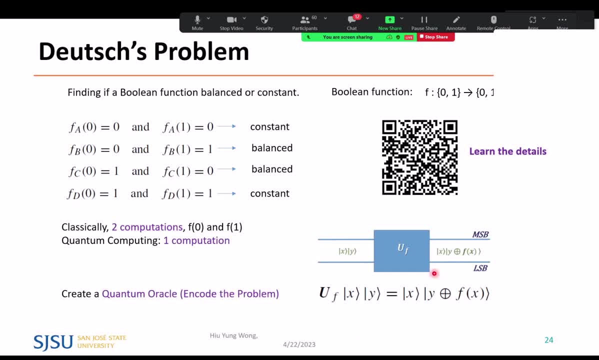 implement the quantum oracle. let's say we can implement. but a quantum oracle again is just like a huge quantum gate. it's a gate, a complicated gate, but it still just tell me, when i have input- x, y, x, y can be 0 and 1- what the output will be. you see, the output is that x is going to cap constant. 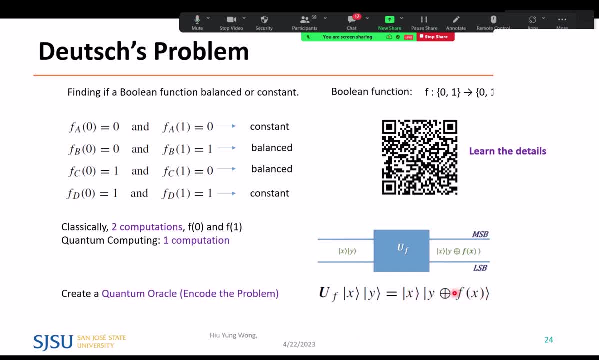 just like a control, not gate, but the output. the second qubits, the target qubits, will become y exclusive f of y, x. so you see that the information of f is encoded in the quantum oracle, but what is f of x? you also see that this oracle cannot tell you because it only 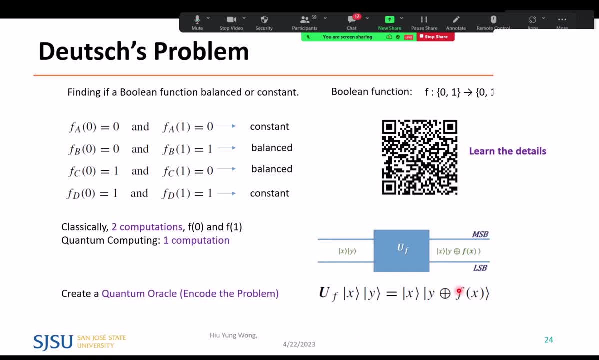 uh, give you y exclusive f of x, not f of x, so we actually are missing some information in order to get this answer. the overall result is that i can find out whether it is balanced or unbalanced, or even over the top, which is what it means, and so you can see that the 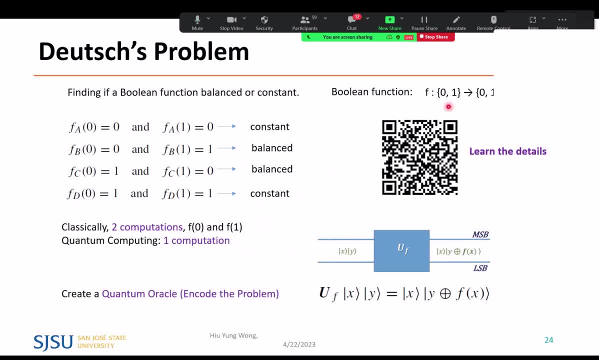 function is much faster when i input zero, let's say zero or one, because f of x is constant. but it is much faster by only using one computation. and it's the same if it turns out that we have many qubits, also only one computation. but i don't know what the function is. i don't know when i input. 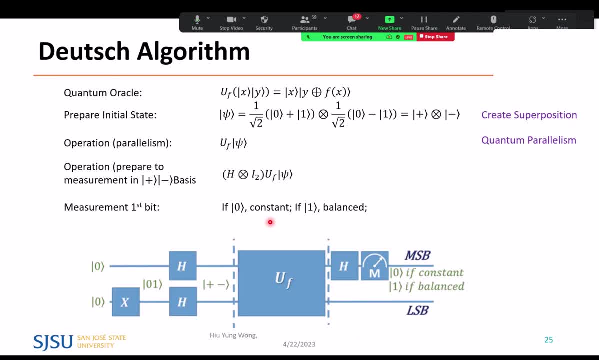 zero, it is going to give me 0 or 1. okay, so this is the old flow of the, the flow of the algorithm. again this. you don't know this if you did not study before. i just want to show you that you appreciate how people construct the algorithm and what are the critical parts on an algorithm, and most of 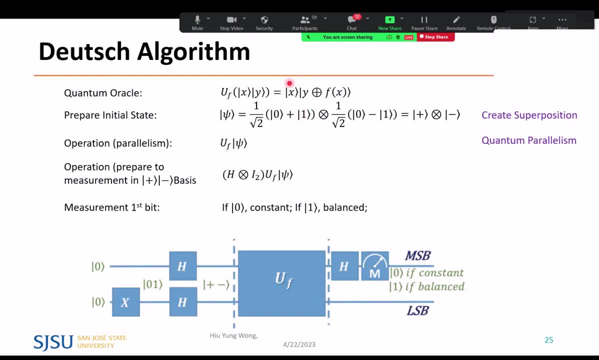 the algorithm are pretty similar. first, you need to have the quantum oracle, as i just told you. you need to encode this f of x into the oracle so that it has this relationship. there are other types of oracle, of course. another thing is i'm going to prepare this in a superposition. i hope you ring. 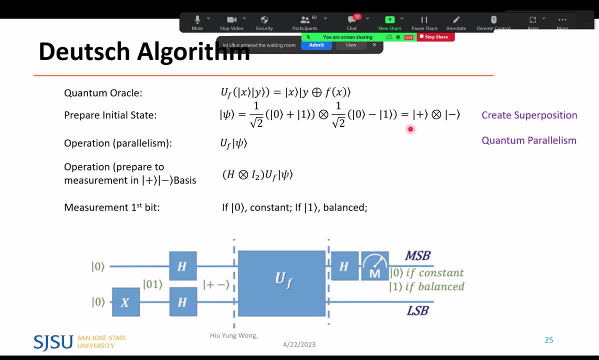 the bell. i prepare it in superposition because i want to do quantum parallelism. i want to have all these states at the same time and then i apply to this oracle, then it will compute at the same time. now, as i told you earlier, i cannot get the coefficient fast, right, because i need to do 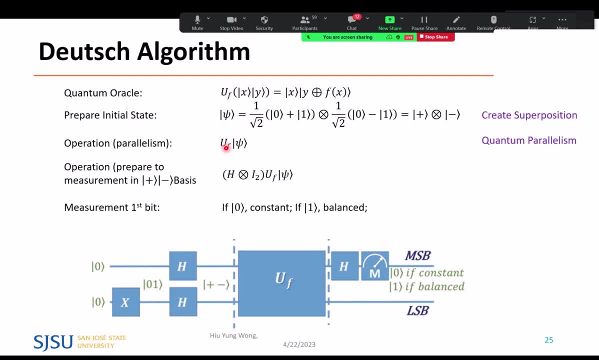 measurement many times just to know its relative magnitude. so i need to do some special operation, which basically is just constructive and destructive interference, so that in this case it always gives me zero at the output if the function is constant and it always gives me one if the function is balanced. 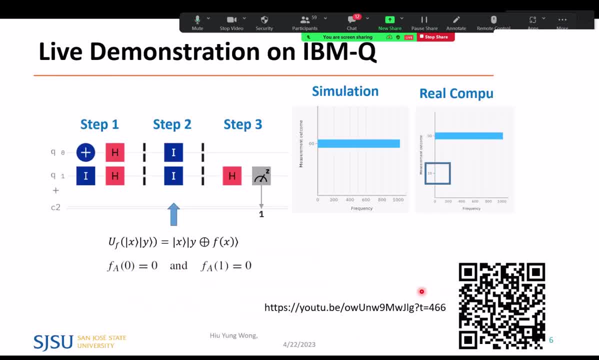 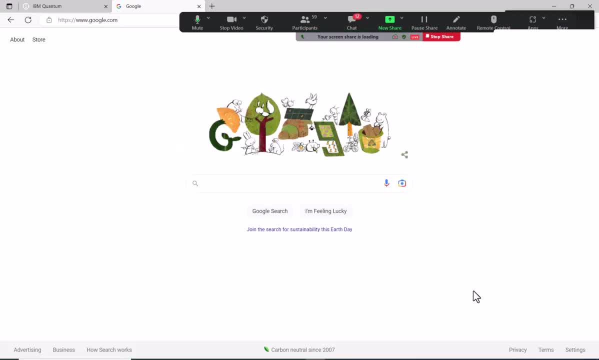 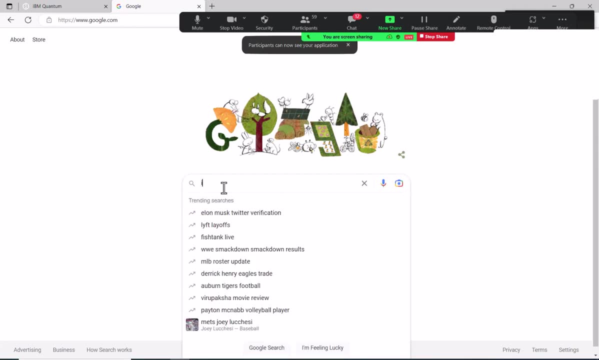 okay, and that is how dodge algorithm is constructed. okay, so let me do a quick live demo. i don't want to waste you. can you see my screen? yes, we can still see it. yeah, so it's called ibmq, i just? i already have my accounts, right? 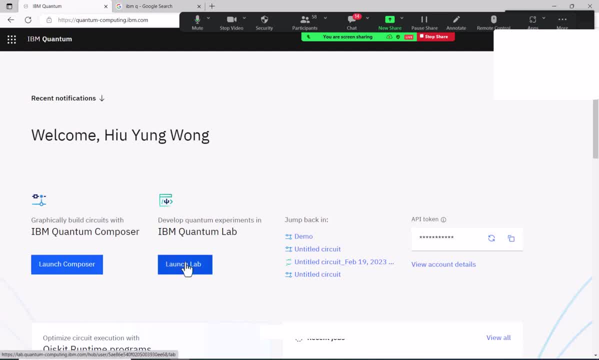 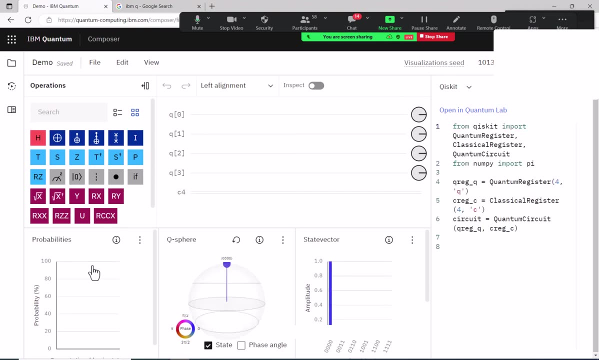 it has two things. one is called lab composer, one is called launch lab. right, composer is the gui. interface is a simple, so we'll do this. the lab. you can use the python programming to run it. okay, so i come to here. uh, this is, you see, the interface. you see, probably you already see some of the gate. 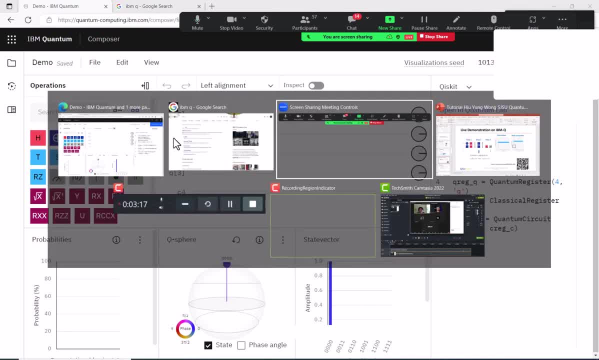 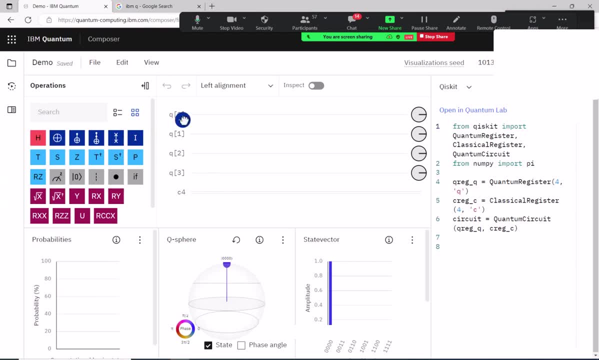 already right that you can recognize some of them, right, and i need to, uh, take a look at my cheat sheet, right? so, just, uh, i'm going to have two qubits. so maybe what i'm going to do is just right click, no, maybe just click, left click: delete those that i don't want, right, and then i'm going to apply. 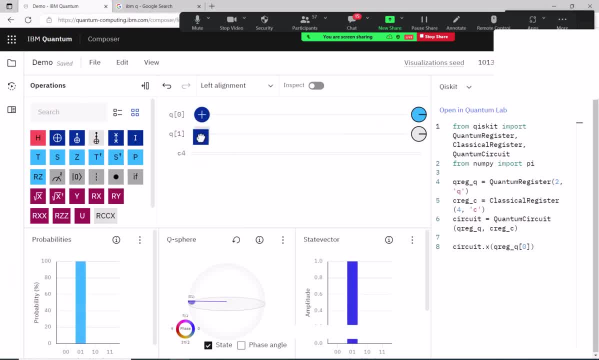 not gate to this and an identity identity gate. identity gate means i'm not doing anything, not gate, just make zero to one and one to zero, and after that i put two hadama gates. the reason is that i want to create a super position. i add this uh breaker just to make it nice. this has no uh function and after that i need to put: 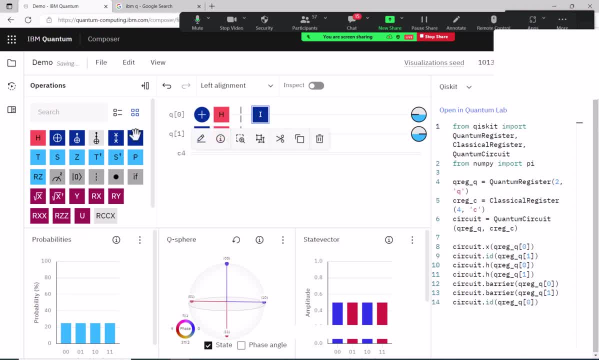 the quantum oracle. now here i put a very simple quantum oracle which is just corresponds to the a constant function when all the output are zero, right, So I don't go into detail to prove that this fulfilled that. but this is just for a simulation purpose. demonstration. 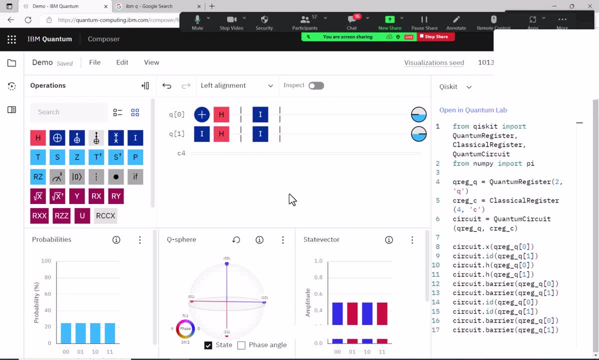 purpose In reality. of course, you don't know what the it's difficult to construct the oracle right. It can take a lot of time to construct. then your algorithm won't be useful. Then I apply a Hadamard gate, as I say, to do this interference and then eventually, 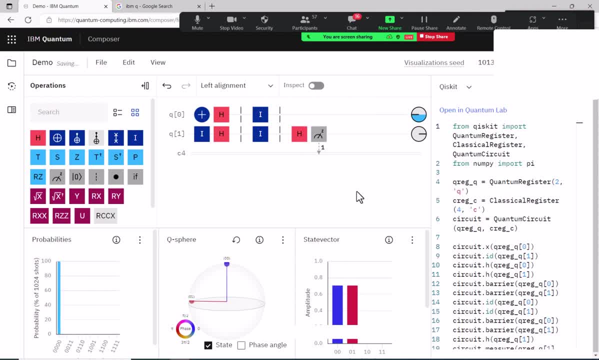 I will do a measurement right, So I'm not showing the slide. but I said earlier, if this is a constant function, then I expect the output to be always zero. okay, Now here it has four classical registers. This is just a register to store your output. So originally. 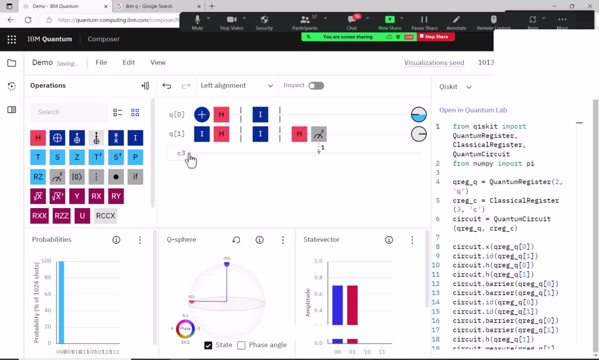 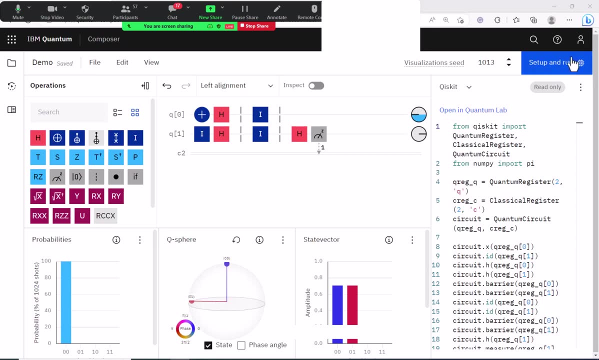 it has four qubits. that's why it has four. so I'm going to reduce it to two, because I only have two registers, right? And then what do I do? I will just submit the sorry. I will just here, go here, set up and run. Now it does. 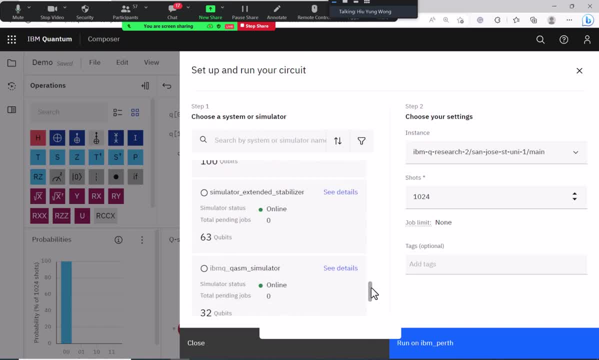 have many real quantum computers. but nowadays it takes a long time. sometimes it takes one or two hours, even longer. So I will just submit to a simulator. This is basically just an emulator using classical computer, right? So I just click on this and then I submit. 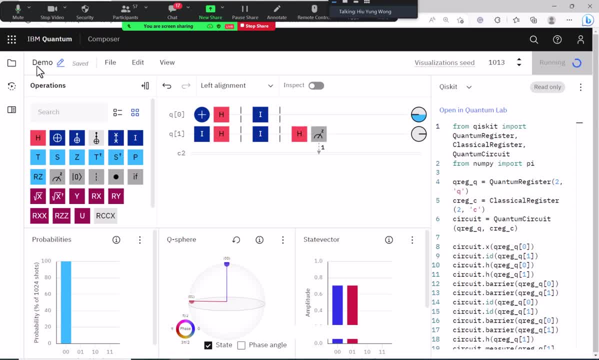 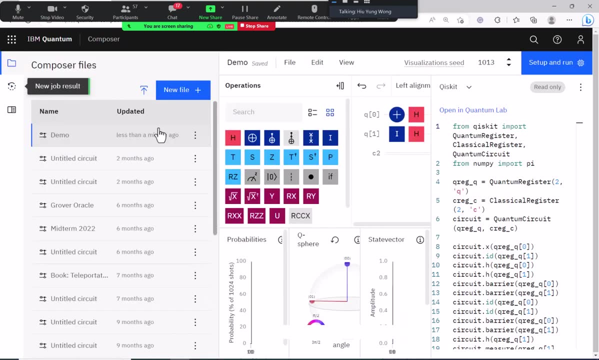 the job, So it may take some time. I don't know what will happen, So maybe I will just show you what I had. sorry, set up and run right. Okay, it has new job result already. This is fast, right, Just so I click on this. It takes some time to load. 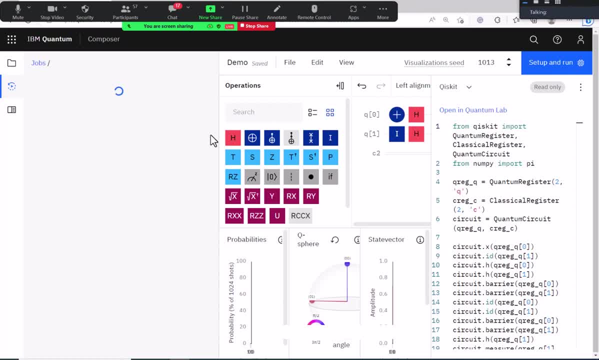 Now let me see. Just bear with me, if it doesn't work in 30 seconds, then I will open my old results. Okay, it has the results. I do want to show you something so you have a better understanding about the quantum computer. Let me see. Oh, Okay, Yeah, Anyway, I will show you in another. 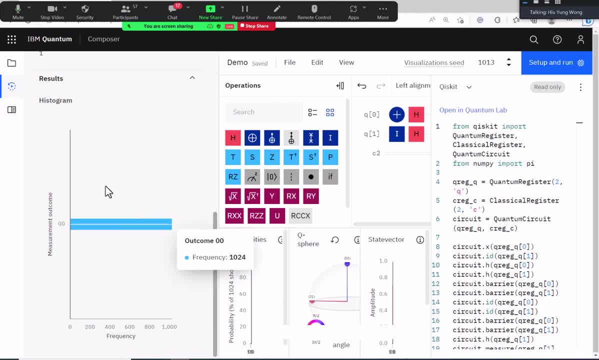 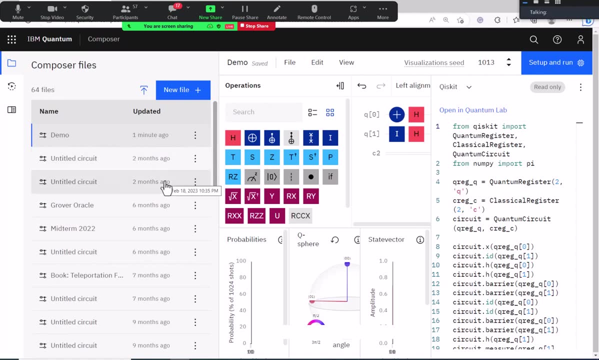 example, because this is simulation. I cannot show you that. Now. this is the measurement outcome. you see, it is all zero. right then we know that this function is balanced. Actually, what I want to show you is the job that I ran with the real quantum computer. 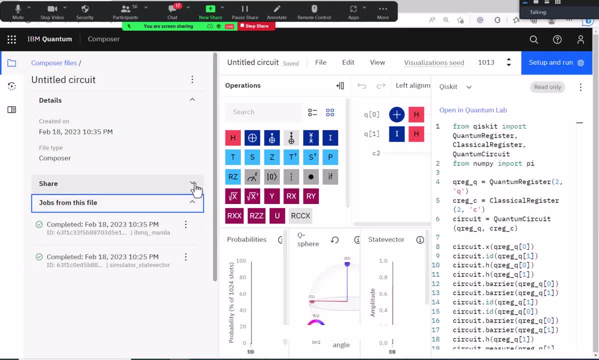 Unfortunately I cannot find it, but basically what I want to tell you is that it will go through a compilation process. So what you are doing here is just a gate, but then you will further compile it to something with higher fidelity, so that it has a more primitive gate, or you can say more primitive. 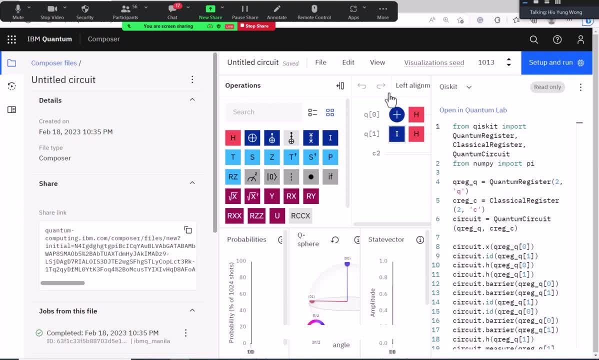 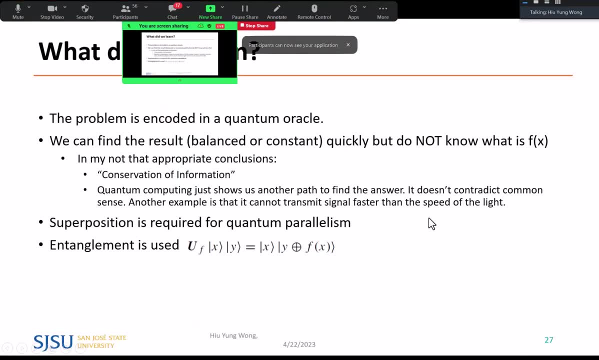 gate, so that you have a higher fidelity. okay, So I will stop here and go back. Can you see it? now I'm on the presentation mode. What did we learn? Can you see it? Yes, I can see the slides. 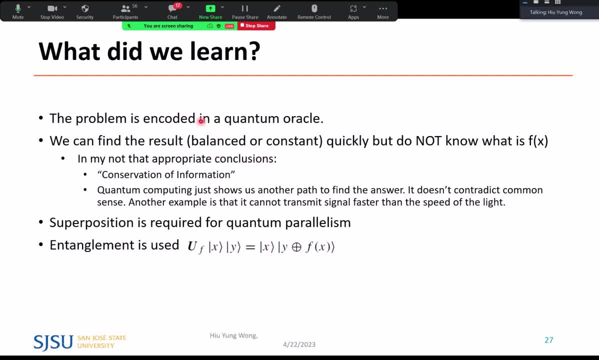 Thank you. Yeah, so basically I already said what we have said: we are encoding the quantum oracle, but this is information, something I want to say. quantum computer is not really something very- I don't know- Unbelievable right. 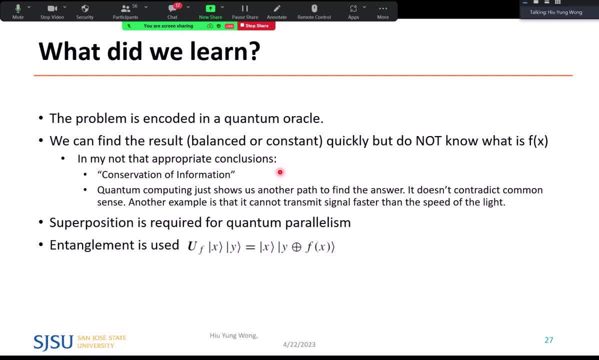 In this example we see that, yeah, I can get the answer quick, but it doesn't mean that I get all the answer I want It is. I feel that it has something like conservation of information for the time you can spend. 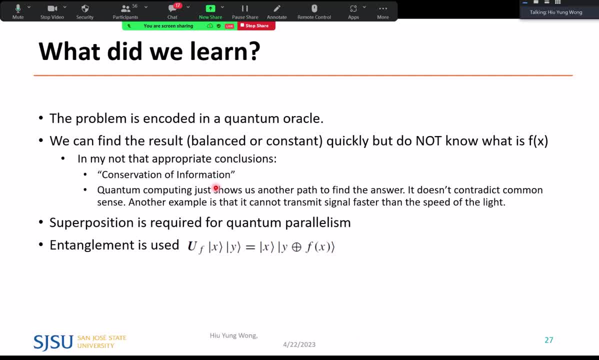 What we are doing? just we give up the details of the function so that we know that which is zero and one right. So I feel that it just show us another path to find the answer, but this is just a hand waving. Maybe the mathematician 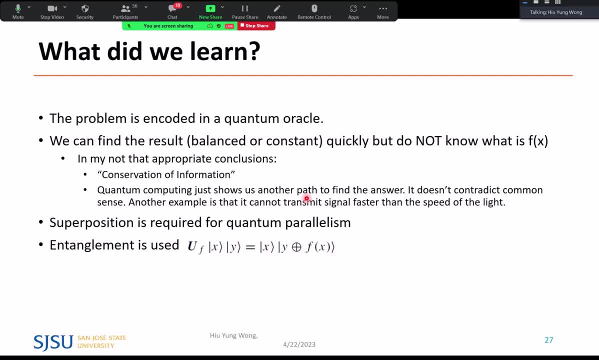 Can prove that I'm wrong. They really have real proof that, saying that the information we can get from there is much more than the classical computer. But the most important thing I do want you to understand, there's a trade off of the information, Okay. 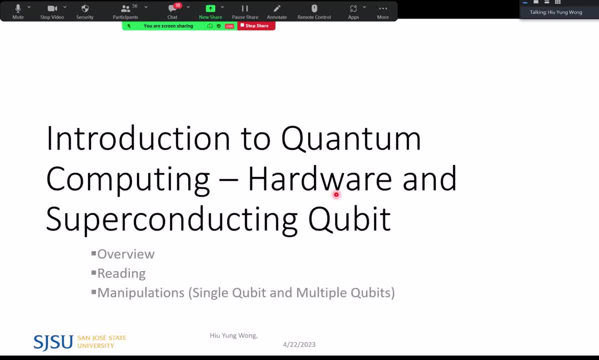 So I'm done with this, Let's go on. Yeah, So we have learned the basics. The algorithm looks very fancy- Right, If they were. But how do we improve? How do we implement in hardware? There are many different hardware. 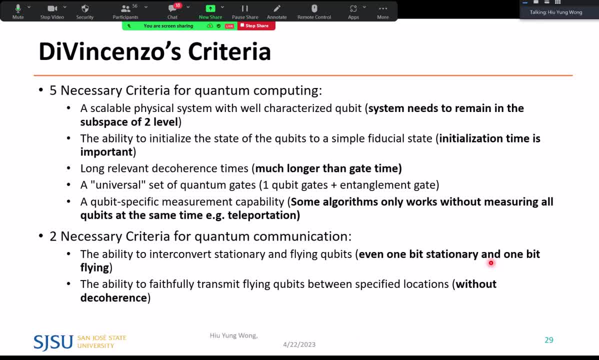 So first we look at this division of those criteria: What hardware can be used to make a quantum computer? First you need to have a well characterized qubit. Basically, what you're saying is that your qubit need to have two basic states: zero. 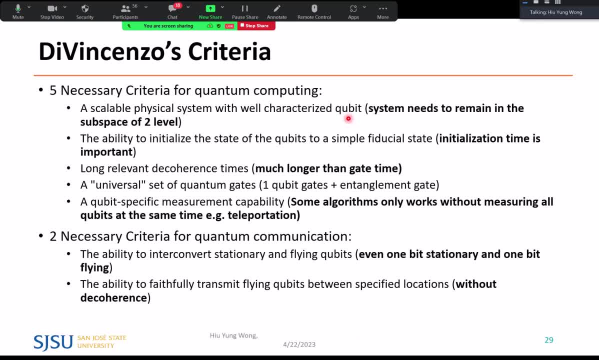 and one. Do not give me more, Because all the physical system they can have multiple qubit. They can have zero, one, two, three, four, five different states. If that happen, you are operating in a higher dimension, higher, more profound qubit space. 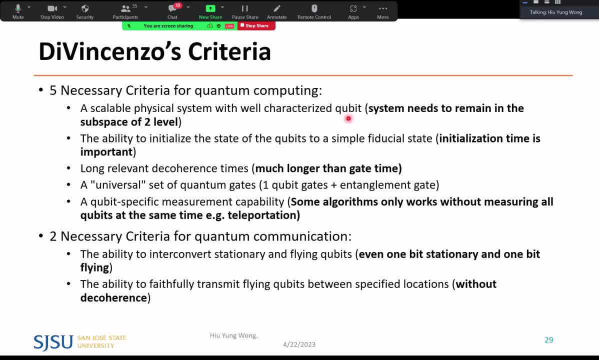 And you leak the information to another space, Right, Then it won't work. Of course you can say you formalize your quantum computer to work on four level. That is also okay, Just like classical semiconductor or logic. Right now we're zero and one. 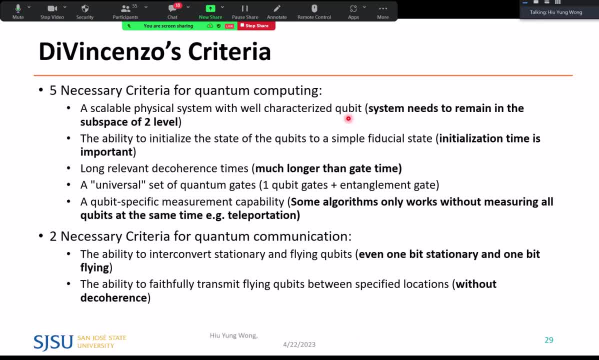 We do have multi-level logic, like even the flash memory. They have three, One, they can store zero to seven, eight states or even more for one bit, Right So? but if we say that only zero and one, then you better have a system that will lead. 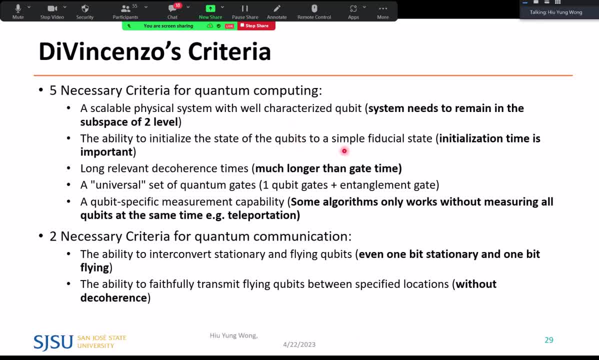 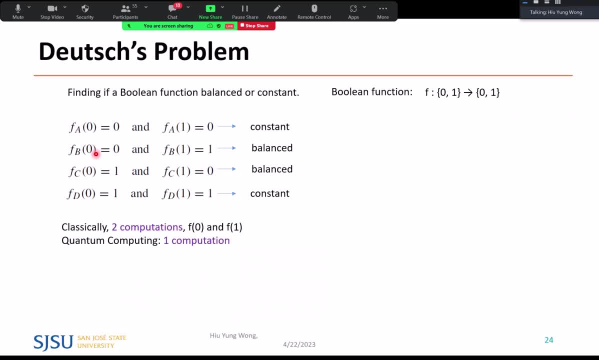 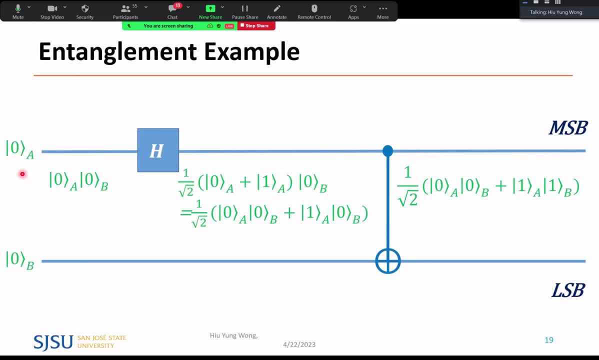 to higher state that because that would cause error. You need to be able to initialize them quickly. If you just take a look at the algorithm I just show you: we, all we initialize it to zero, for example. zero at the beginning. 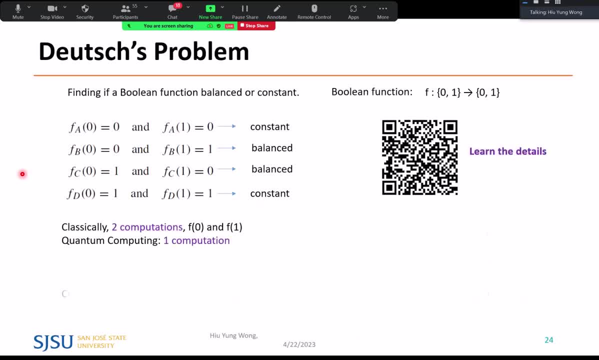 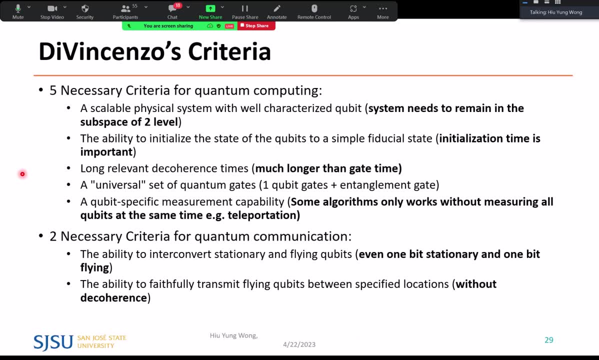 And that is the best way to start the quantum algorithm. Okay, And so you should be able to initialize it. If your system is going to take one minute to initialize a qubit, it's not going to work, because there are many algorithms you want to initialize very frequently and many times. 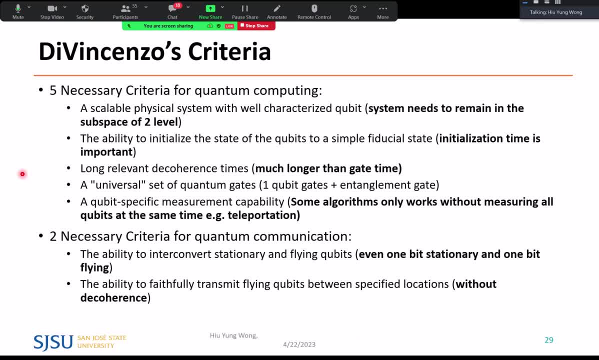 And also meant for like last time. we say we need to run many times to get the answer, So you need to run it initialized many times And then you have to run it again, Right, And then you will have a problem, right? 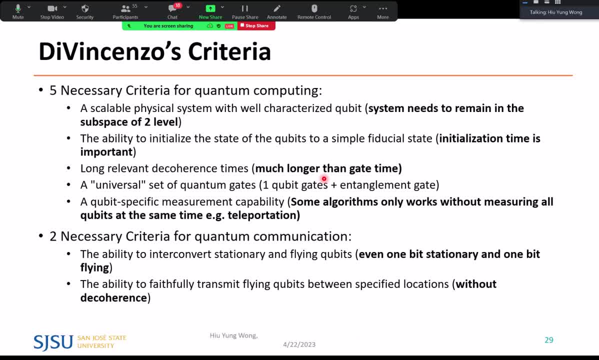 Long coherence times When you are at zero. you better stay at zero At one. stay at one. Do not change to other states before I finish the computation. So you want to have coherence times longer than the gates time? right, You definitely should be able to do one qubit gates and entanglement gates. 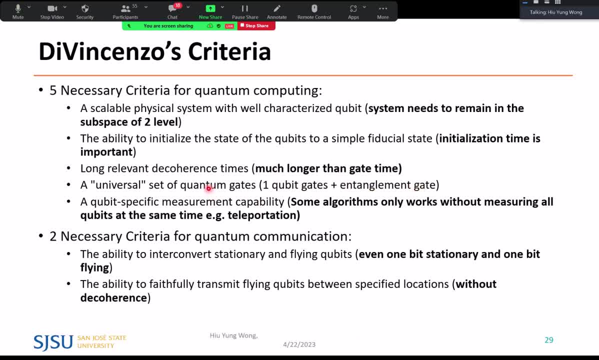 With this, then you can do most of the algorithms. Another thing is that you should be alive. Allow them to measure individual qubit. Sometimes the whole system needs to be measured. then it won't be useful. Just like the spooky action I just mentioned to you. I measured the qubit on the earth. 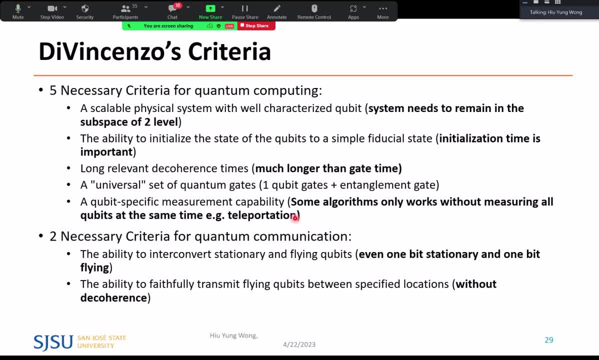 If your system needs to measure every qubit at the same time, it won't work. For example, something called quantum teleportation will not work if you need to measure them all at once. If you want to use quantum communication, you also need to make sure that the qubit is. 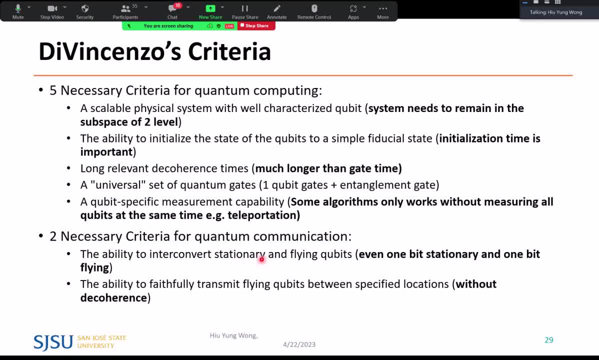 flying, So you need to be able to interact with the stationary qubit, And also, when you are flying you need to keep the coherence right. But we are only talking about quantum computer here. So how do we implement the qubit? 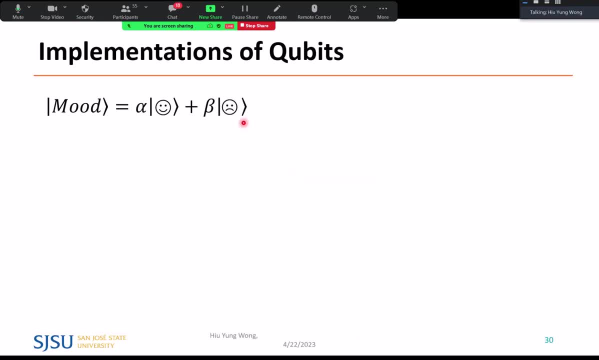 Well, as a joke, it can be a superposition of happy and sad. You ask me how's my mood today? I may say, oh, kind of happy, kind of sad. right, But not reliable In reality. what we can do is 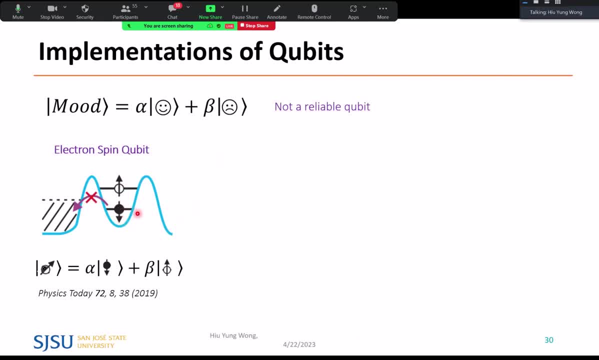 How about spin qubit? It can be spin up, spin down, then they have two different energy levels in this quantum dot And then you can form a superposition of these two qubits. You can also use photonics. This is just a waveguide and I did not draw it. 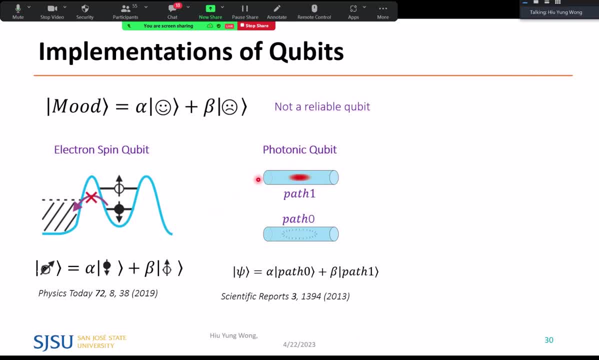 You shoot a photon, one single photon, and they are symmetric. So where is the photon? In quantum mechanics, it is a superposition of these two paths. It came on the top and the bottom path. That is the superposition. So what is the superposition? 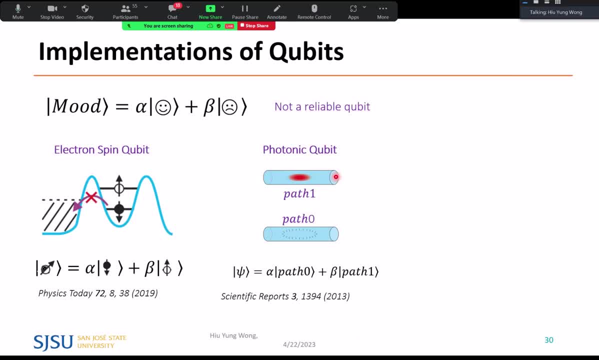 When you measure it, you can either only find it either here or here. You cannot find it at both right, Because I only have one photon, That is, the collapse of the wave function. The one that we are going to talk about is the superconducting charge, qubit. 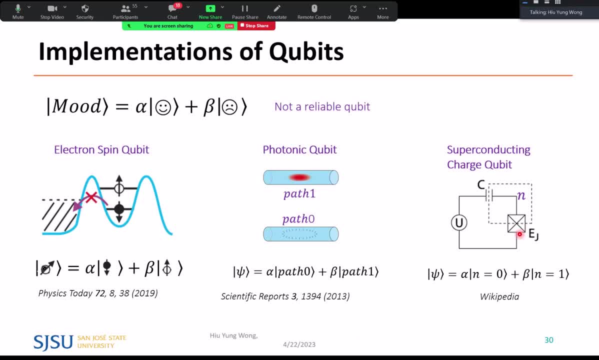 This is something called Josephson junction. Josephson junction is just like an LC tank. If I add a capacitor- large enough capacitor, it also has its parasitic capacitor. It's just like an LC tank. It's just like an LC tank. 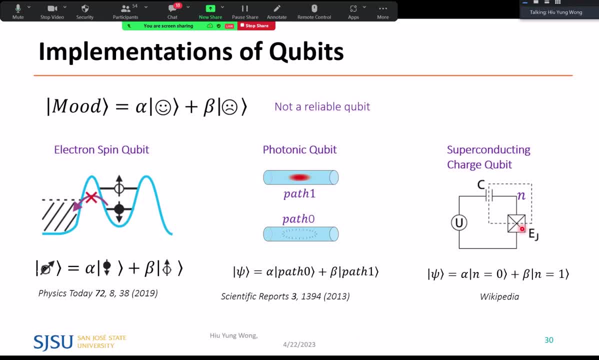 But it has long linear inductance. Because it's long linear. that solves the problem of equal spacing of different levels in a simple harmonic oscillator. I just told you that to be a quantum computer you need to confine it between zero and one. 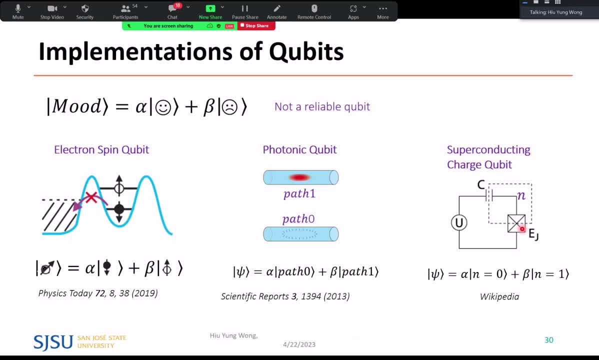 state, You cannot lead to second state. So if we have different spacings, then we can confine it in zero and one. And what it does is this: It has a capacitor here. This forms an island. In this island, you can have zero or one extra pair of cooper pairs. 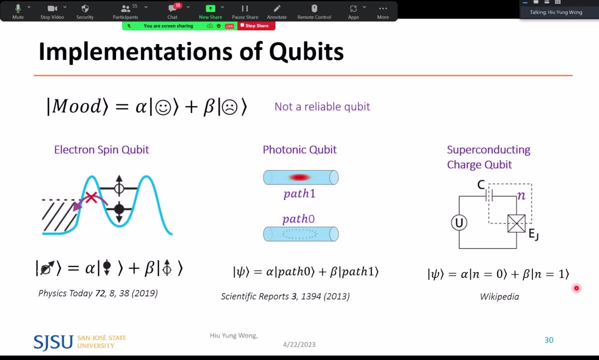 Cooper pairs is a pair of electron that occurs at superconducting state. We don't need to go into that details, But it's just a pair of electron. They work together, So treated as a new particle. So I have one extra, or zero extra particle here that represents a qubit. 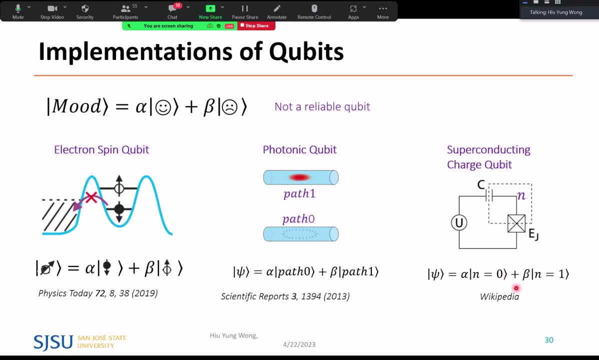 And, of course, can be a superposition, because it's quantum mechanics. i have a linear combination of zero extra and one extra cooper pair. okay, now both. no matter what you use to implement- maybe not for photonics- they only have very small energy difference between the zero and one state. 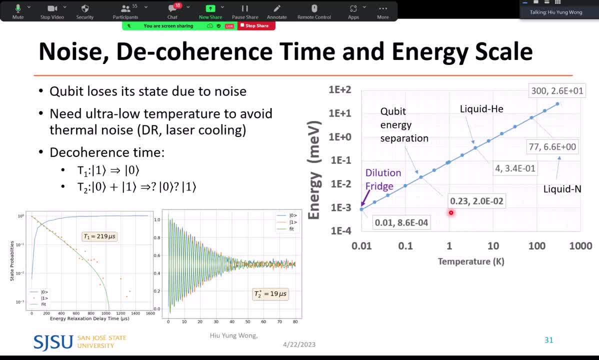 and because they interact with the outside world, they can lose their state due to coherent decoherence. on the right. i'm showing you the scale of energy. scale as a function of temperature. for example, at 300 kelvin is about 26 millivolts of thermal energy. we can cool it down by liquid. 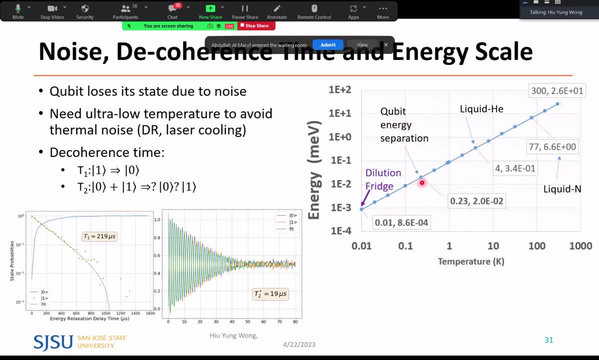 helium to four kelvin, but a qubit separation is only in the order of what? 0.02 mini kelvin, very small, is equivalent to 0.3. so sorry, i say the wrong thing. the energy is 0.02 mini ev right correspond to 0.23 kelvin. in order to make it work, we need to cool it. 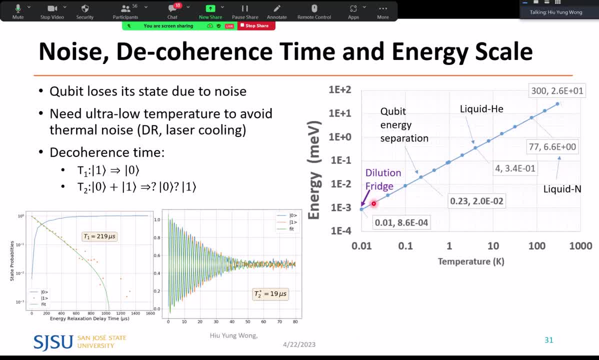 down so that the environment is cool enough, for example in direction refrigerator in the order of 10 minute kelvin. then you have the thermal energy at least 10 times less than the qubit separation, so that you won't be affected by the thermal energy. so you have a 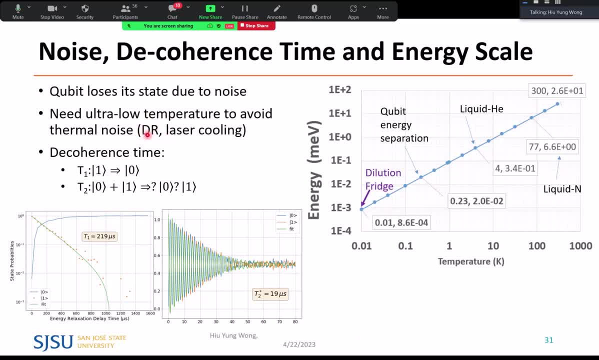 longer coherence time. you can use direction refrigerator, dr or laser cooling, for example in the trap iron. so what is the coherence? for example, i may be in the one state and i keep. i try for different time. so here i did. this is a real quantum super contacting quantum computer. 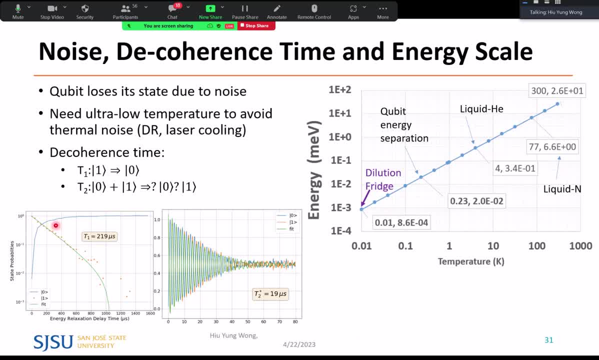 experiment in we did in livermore national lab, the. when you wait for a long time, when you measure it again, you say that it starts decaying to zero. the probability of fighting one becomes less and less. this is so-called t1 coherence time- only in the order of 219 microseconds. 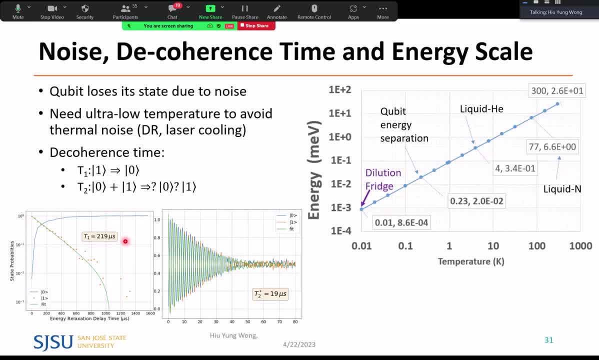 so you can imagine, your gates need to operate way faster than that, maybe, uh, 0.5 microsecond, so that you can have enough operation before it decay okay. another thing is the so-called t2 decoherence time. it is saying that i start with a superposition. it is still in superposition. 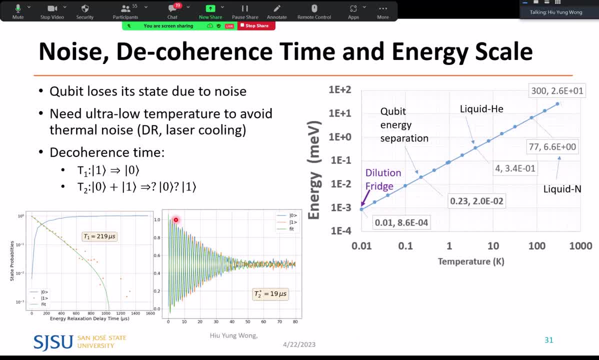 but it lose the phase gradually. usually it is much shorter than the t1 time, as, as this is a oscillation- uh, i can, i won't. i don't want to have time to go into detail, but that is the way to measure the t2: we bring it to the superposition and then rotate it back to non-superposition, and 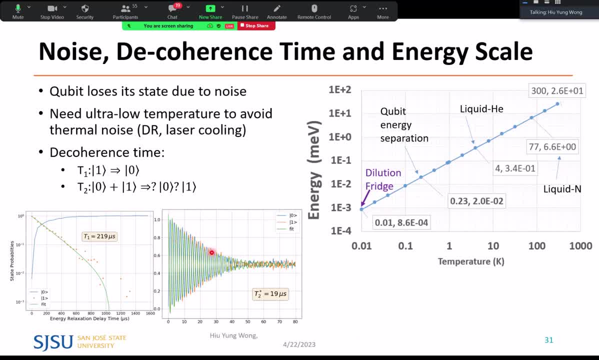 measure the zero and one states it will oscillate, but anyway, the envelope determine is the coherence time right. so you need to be less than t2 because t1 and t2 are all there at the same time. so you need to be much less than t2 for your qubit to work. 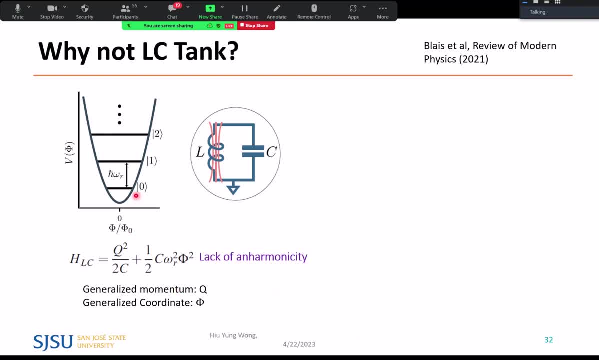 so i just told you: uh, we can actually use the lc tank to make a qubit, right? if you do some quantization- right circuit quantization- you will find that it behaves like a simple harmonic oscillator. you have zero extra electron, one extra electron, two extra sorry photon. zero extra photon. 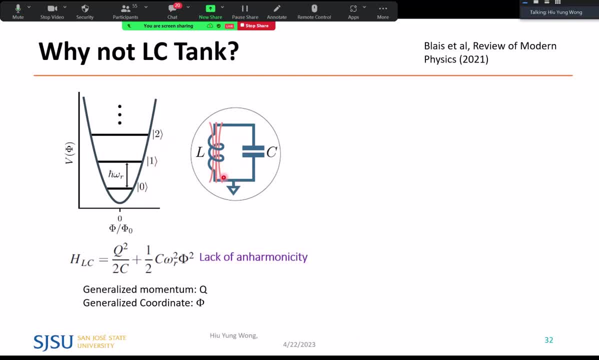 one extra photon, two extra photon. you will feel surprised. why you're talking to me right now? because it will know less than you know more than any other��ve IBMァ, I'm eggs. see you in the next, me between devices. why you're talking about photon. remember electromagnetic wave photons are 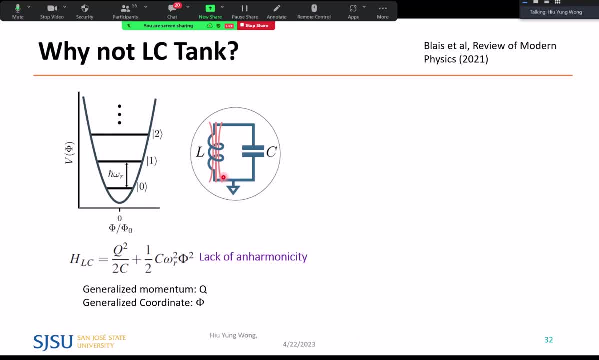 electromagnetic waves. that's why we call it photon. right, so everything is governed by Maxwell equation. so zero, one, two photon in this LC10. the problem is that they have equal spacing. so we see that lack of and harmonicity. when you have equal spacing, then apply a pulse, you go to. 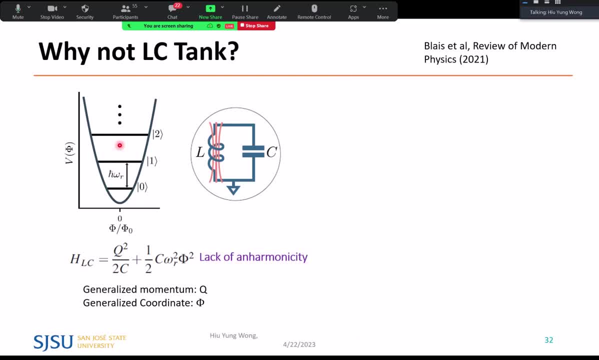 one, apply another pulse. you won't go back to zero, because you may go to two, then screw up. that's why we use the simple harmonic. uh, use the Josephson junction. here is something called transform, we pair, we have a parallel capacitor. in this case, you see, the energy separation becomes. 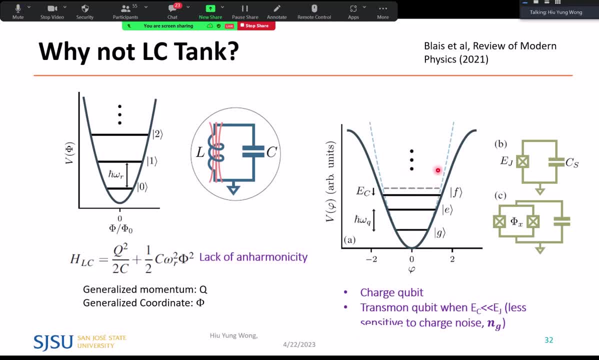 smaller and smaller when you go up right, so I can confine them in the zero and one state of course. now, this is photon, this is like extra cooper pair for for this qubit right, and here it has two important quantity. one is so-called the ec, the coupling, uh, the capacitor, the capacitive. 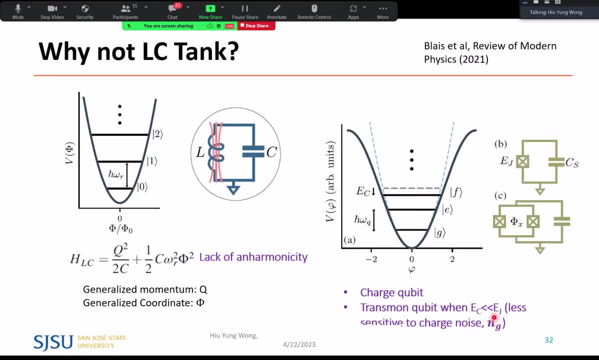 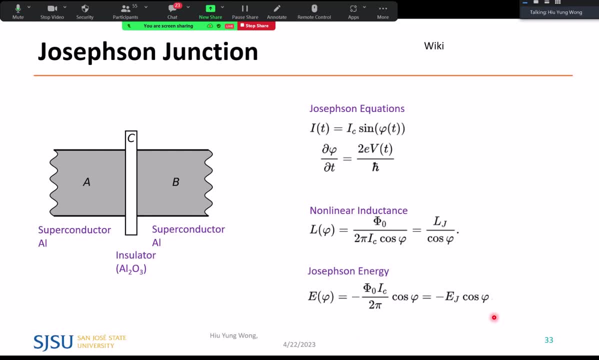 energy here due to this capacitor. another is josephson junction energy. and what is that? don't worry about the equation. i showing you this. just want to show a few important concept. josephson junction is a very simple device, a metal insulator, metal just a capacitor. but because we cool it to 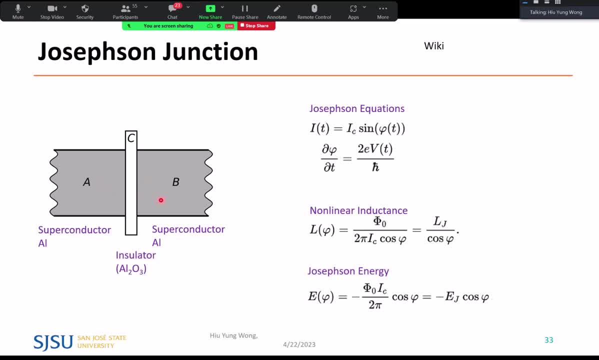 very low temperature. it becomes a superconductor, insulator, superconductor, that's it. the special thing about this is that it has a constant current or its current depends on the phase difference across it. we did not discuss this, so i'm sorry if you don't- uh, if you don't really. 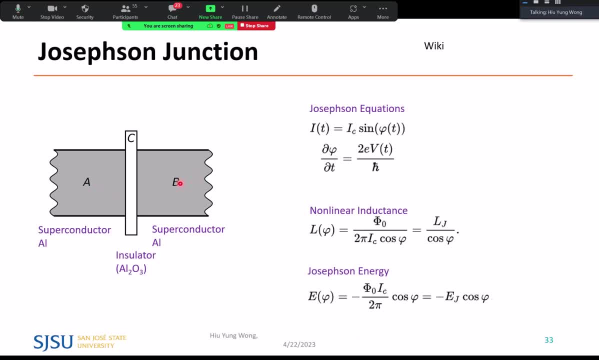 get this because it needs a lot of explanation. but there's something called phase for this, uh, quantum object, for this cooper pair. they have a phase because they are the wave function. the phase difference determine how much current going through and the phase will change if you apply a voltage. so basically, even you have zero voltage, 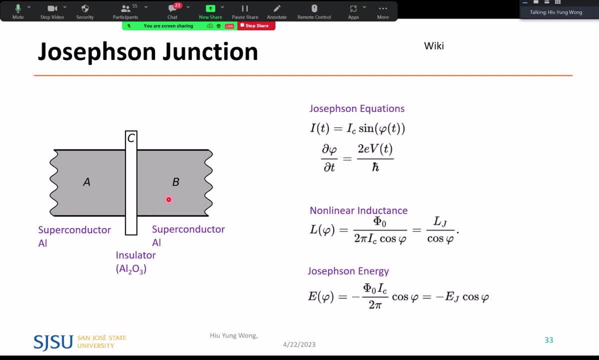 but you have phase difference, you get current. you don't have this in a regular resistor, right and then, and that is because they're superconducting- even you don't have voltage. you expect a constant current, keep going through. okay, so that is the so-called josephson junction equation, and it has long linear. 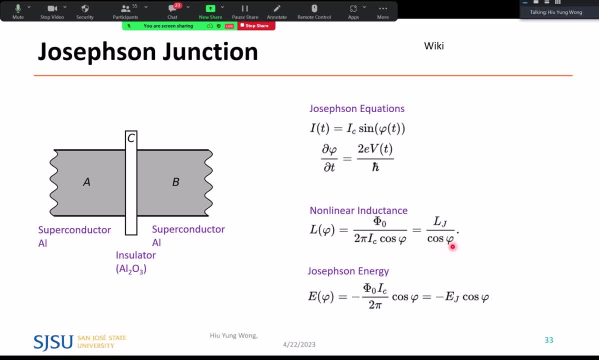 inductance. that is what we just said. okay, it depends on the phase. the only message i want you to remember is that its inductance is non-linear. that's why it makes it a good qubit. it also has the associated energy, because it's an inductance right. an inductor has energy, a capacitor has. 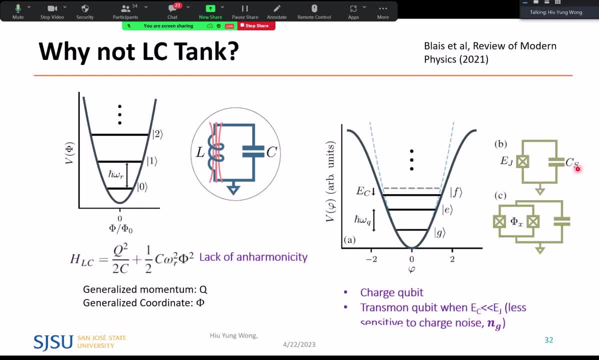 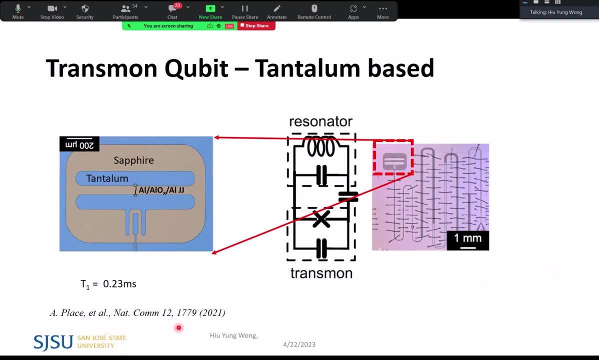 energy. so that's why we have this e, c, capacitive energy, and also ej, which we call it josephson junction energy, but which is nothing but just the inductance energy that it has. here shows the layout of a transformer from this paper. this is the ic layout. you look from the top here the gray one, adjust the insulator, the substrate. 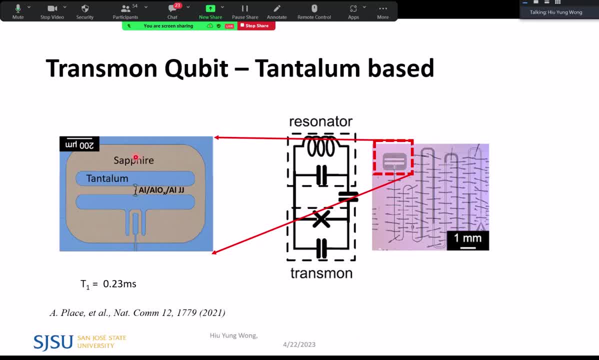 sapphire insulator, the substrate, just something to hold the device. this well tiny thing you cannot see is the josephson junction. aluminum insulator, aluminum, that's it. they form a junction there. that is the whole josephson junction. very simple. but they also have a large 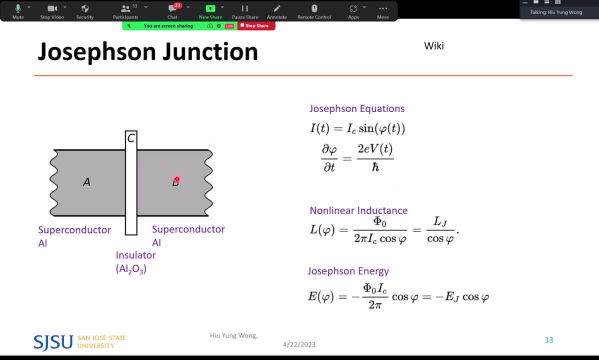 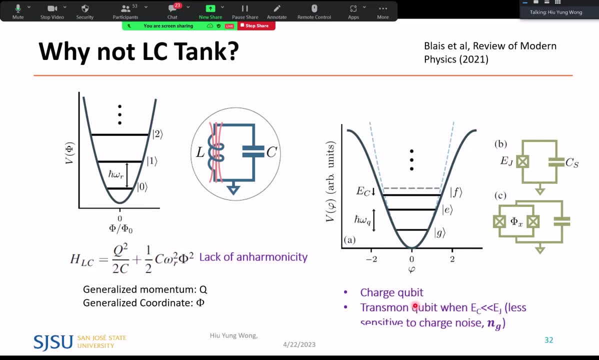 capacitor in parallel, parallel with it. this is tool for this structure. i have josephson junction. i have a parallel capacitor because you want to form something called transmon qubit. a transmon qubit has a large shunt and it has a large shunt and it has a large shunt and it has a large shunt. 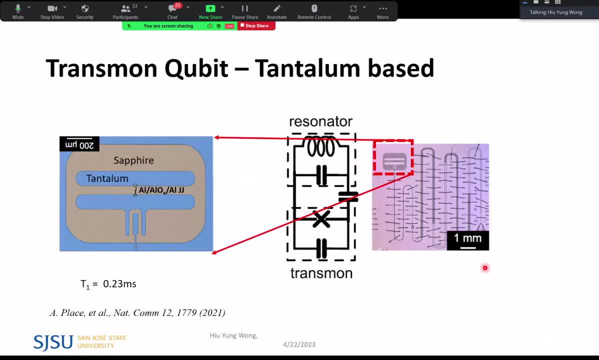 capacitor, for some reason. i will explain later. and this is, this is the qubit already. and i said earlier i don't need to form the gate because i'm going to put the qubit here and then i have a transmission line going all the way to a port. then how do i apply? operate on this qubit? i apply. 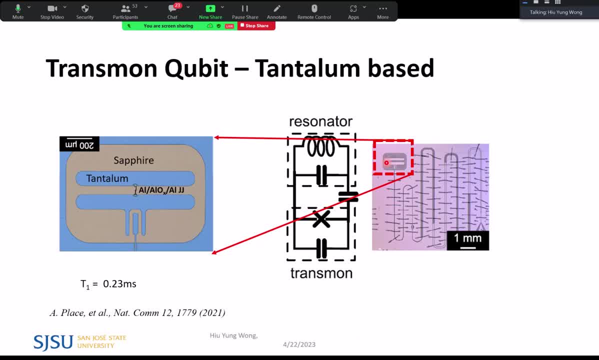 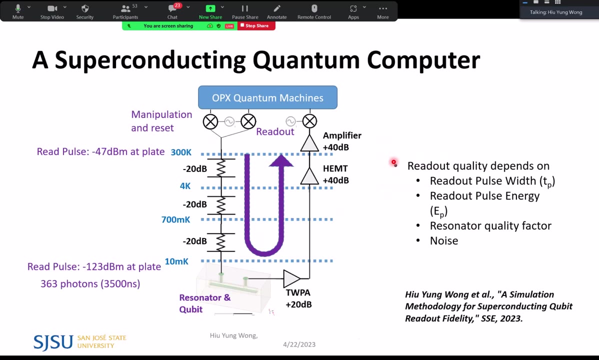 a gate pulse, then the state of this josephson junction, which is a linear combination of zero and one extra cooper pair, will change. the alpha and beta will change, and that is how we uh operate a qubit. okay, now this is the chip, but then how about the whole system? here shows, uh, one of the work we 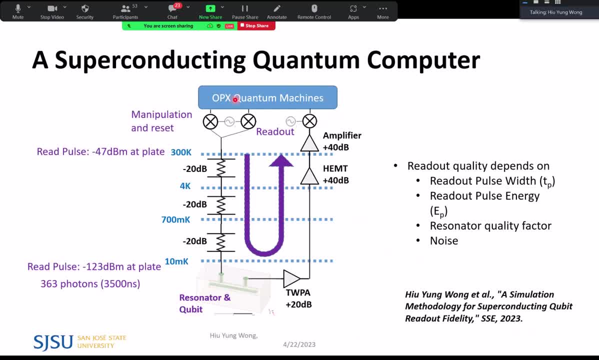 did earlier from this paper. uh, of course it's not about this dump is about the study of the readout. but here shows the uh how a quantum computer is made today. it occupies a whole room, super big, because first you need to have this server from a company called quantum machines. you can have yourself what it. 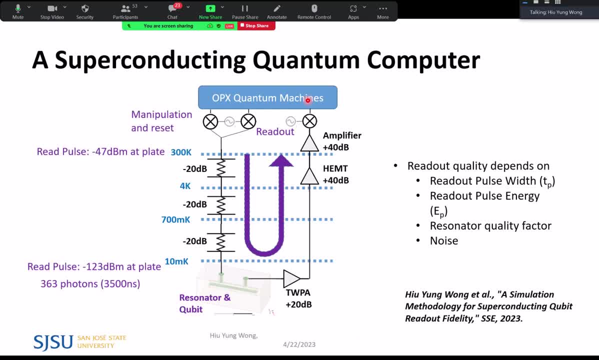 does is keep generating pulse, very high speed pulse, and based on the readouts it generates other pulse. this microwave pulse will get to the mixer to bring to the right frequency and they are at 300 kelvin. then we will go through attenuator to filter the rate of the pulse. 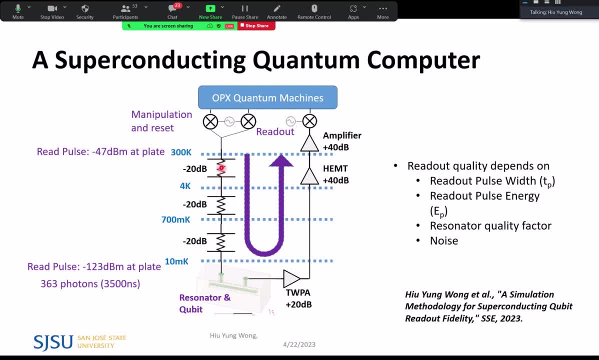 noise. to uh, make them the to reduce the thermal noise. keep going: 300 kelvin, 4 kelvin, 700 minute kelvin, 10 minute kelvin. so this is in the direction refrigerator i just mentioned, and here we sit, a resonator. this is different from this one, it's a 3d resonator, but you see that it's just the same. 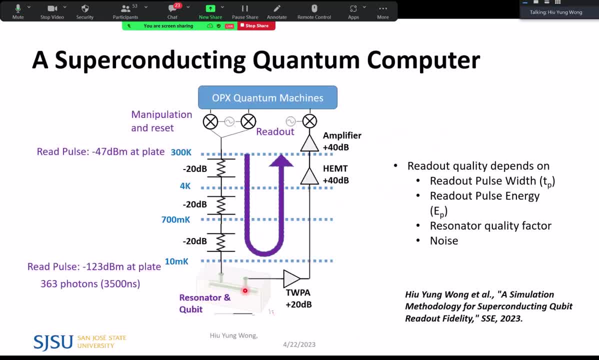 as this circuit and inside the resonator, which has a very, very tiny qubit that you cannot see here. the the pulse we should in is negative 47 dbm, very small. when you get attenuation and reach the resonator, you only have about 363 photons, right, if you make it smaller, so they're accountable. 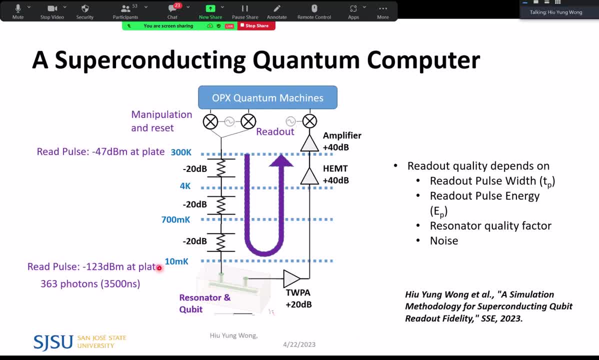 that's why they're very sensitive to noise. so in this setup we are showing the readouts, we shoot the pulse here and then we try to read the pulse, and you need a quantum amplifier which add the least noise to it, and then you have different stages of amplifier to see the signal right. so you see, a quantum computer is really nothing but. 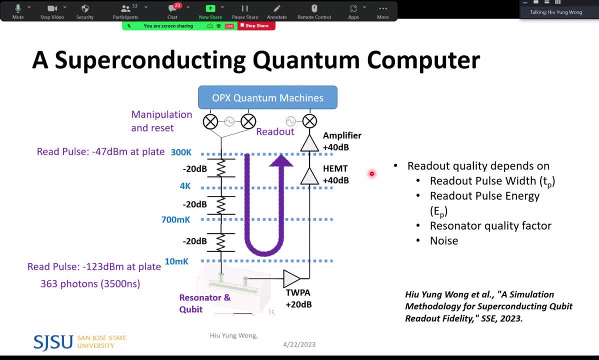 99 percent: classical electronics, cryogenic electronics, fpga, high-speed electronics, control theory, error correction, mechanics and direction refrigerator, and only this part is qubit. okay, so if you're electrical engineer, you're engineer, you should consider to go to this field, because without you quantum computer is not going to work. okay, so here i want to talk about 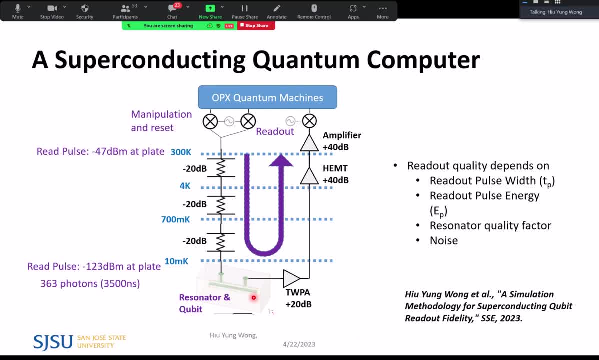 how we read out the quantum computer. so, as a initial introduction, the way we do it is that we shoot the pulse to here. this is a resonator. we were going to detect the pulse. depending on that way to do it, oneề you need to ignore the wave. we were going to detect the pulse. 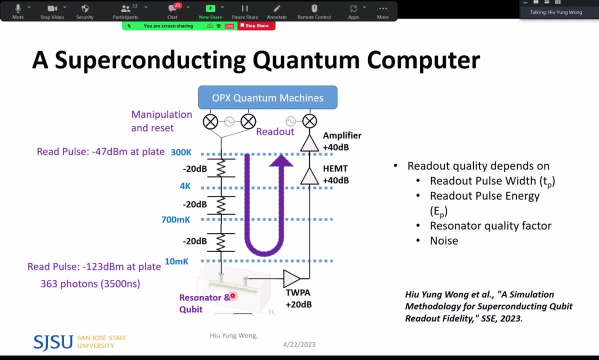 the way we hit inter. different frequency is equals the result. We can read out the pulse that braucht. want you read out the picture you let the Houston proces Teen EN is the function of kidd ready with some depends on the resonance frequency. We will have the largest amplitude when the resonance frequency 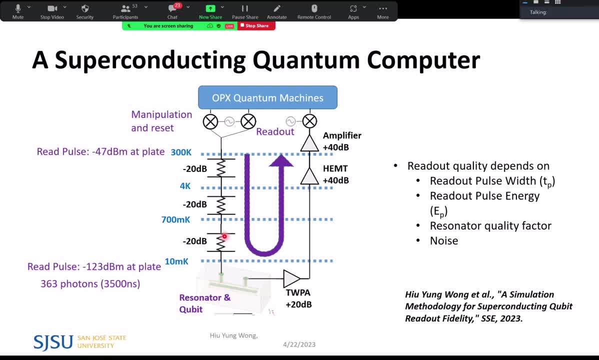 meets our pulse frequency, okay. But when you have a qubit at zero and one state, it's going to change the resonance frequency of this system. So if it is one, resonance frequency may shift to lower. When it's zero, it may shift to higher. And that is how we read out the qubit of a superconducting. 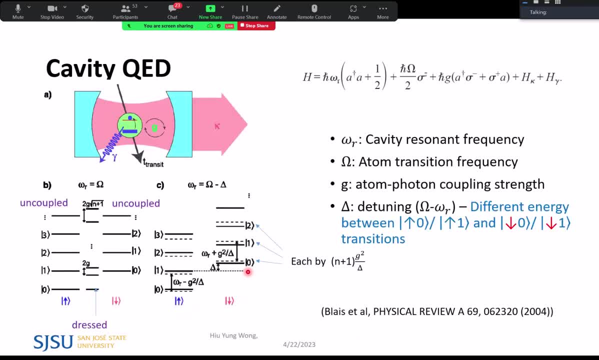 qubit. Because of time, I will just quickly go through this line. Don't worry, because it's impossible to understand if you did not study before. But the message I want to tell you is that there's something called cavity quantum electrodynamics. That's what physics people have been. 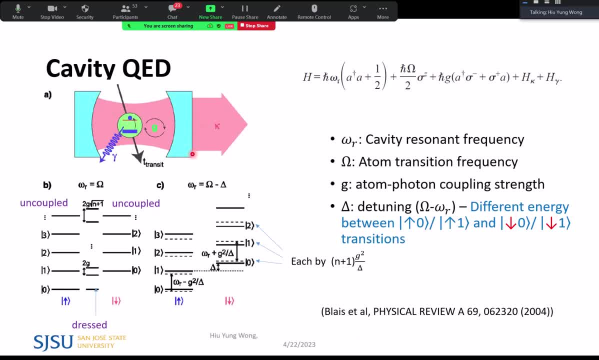 doing? They put an atom here in an optical cavity. This atom has two level system And the optical cavity also can contain one, zero, two, three, four photons And they interact with each other. That is the so-called Hamiltonian. 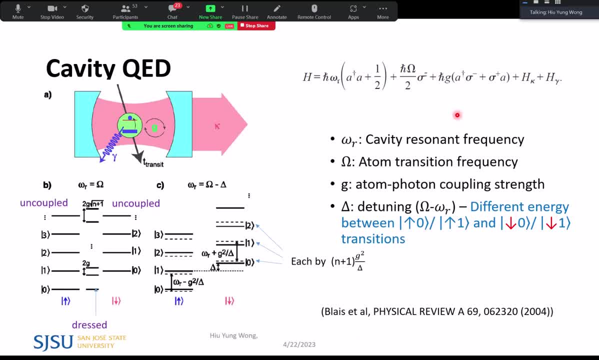 describing the interaction. But don't worry about this. The most important thing is that is saying that you, I can create, I can excite the atom to a higher level by absorbing a photon. The atom will emit another photon by going to a lower level, So that is a cavity that allow us to. 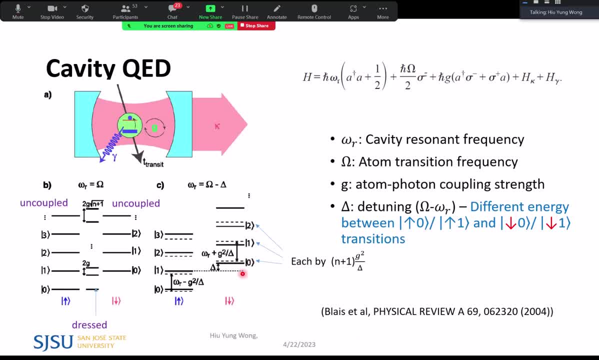 distinguish the level of this atom by shooting a laser pulse to here, right? So, although I did not plan to talk about other quantum mechanical architecture, this is one of the possible qubit that you can do, And it's not similar to trap iron, right? So use the atom as a qubit. This is one of 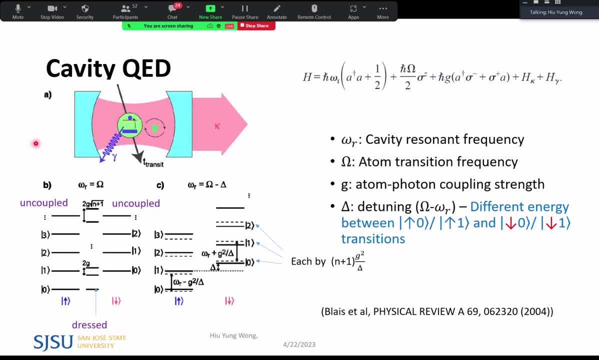 the possible qubit that you can do, And it's not similar to trap iron, right? So use the atom as a qubit And use the laser pulse to probe it or to manipulate it. There are two frequencies: One is the cavity resonance frequency, One is the atom transition frequency, And they also have the 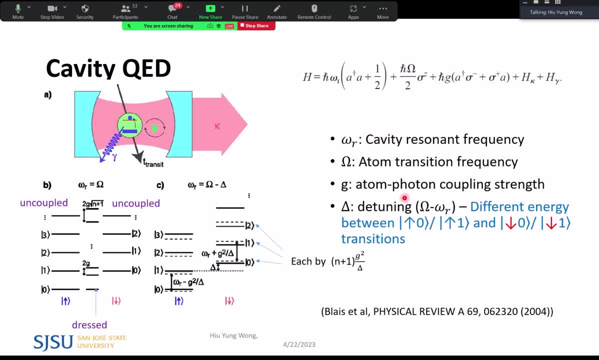 coupling string between them, right. When the two frequencies are different, we say there is a detuning, And this is important so that when this atom is at different level, it's going to change the resonance frequency of this qubit, And when this atom is at different level, it's going to 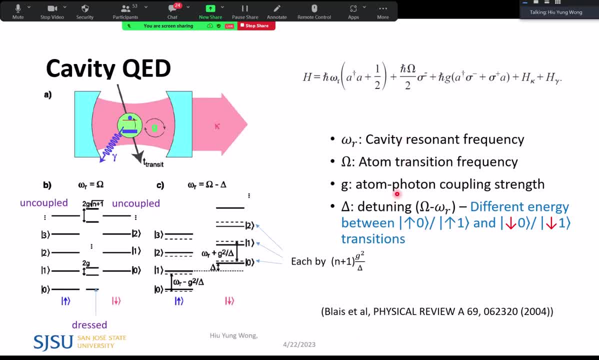 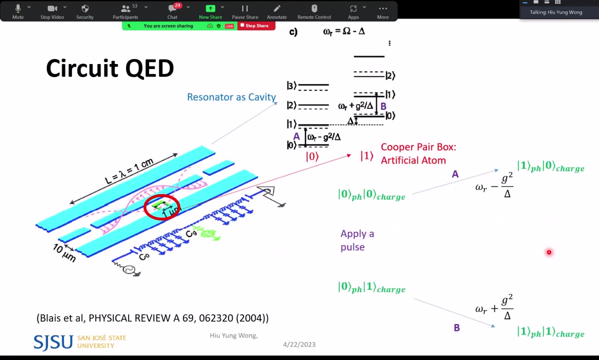 have a cavity overall. If there is a detuning, then you are going to have a different change of these two levels As a result, when your atom is at zero and one state, your overall frequency will shift. This is confusing. I know I did not explain well, but this is just to bring you to. 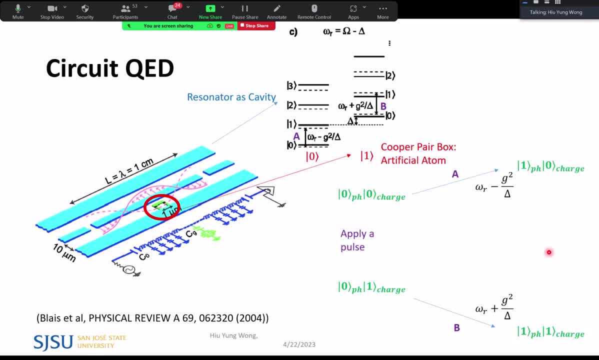 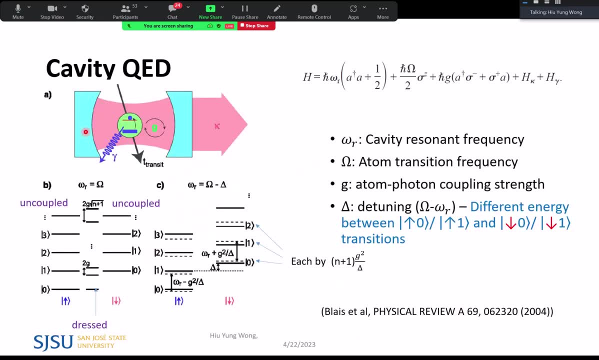 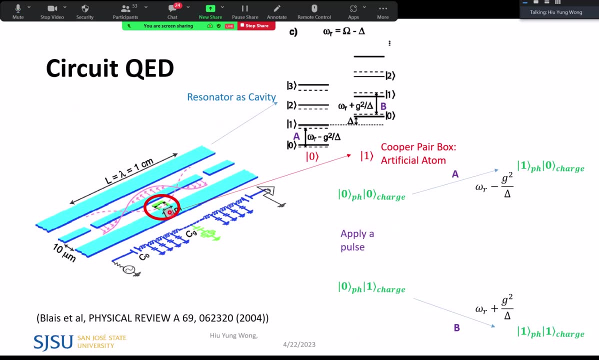 our superconducting qubit. I just want you to understand that. we lay out the chip, we can lay out a resonator. This is the cavity, Just like the optical cavity here, two lengths here, And it's coupled to a superconducting qubit. This superconducting qubit has two levels, right. 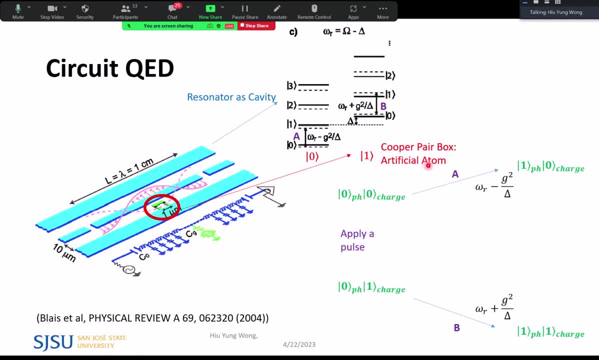 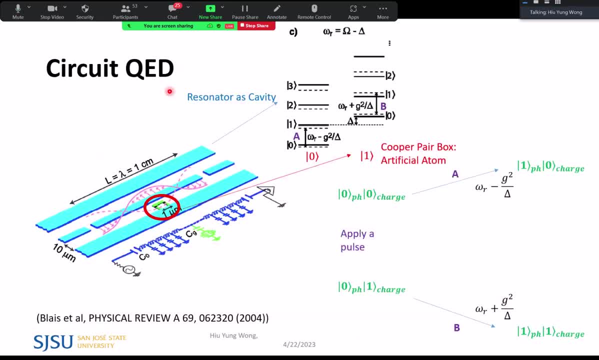 Same as optical cavity but just different wavelength. So I can have a state that have a zero cooper pair and then have zero one, two, three atoms, like this right Photons. So I have zero photon or zero charge. Or I can have one cooper pair but zero one. 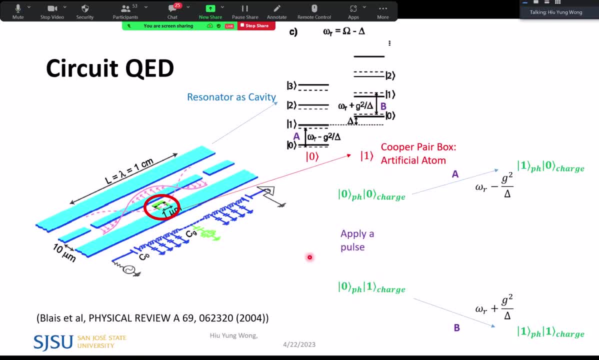 two, three photons. So I have zero photon and one charge- How do I know whether it is zero? and one, And that is what I'm talking about. So I have zero photon and one charge. So I have zero photon and one charge. 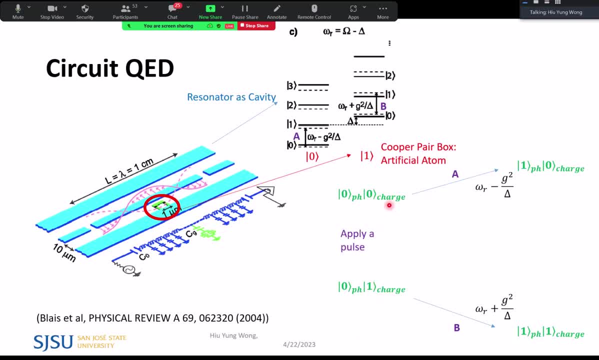 What I try to tell you earlier. the state of the atom is going to change. You see, this omega R minus G2 over delta change the level of exciting of adding one photon to the system. If you have zero charge or a zero cooper, pair the energy you need to excite or to include one photon to this. 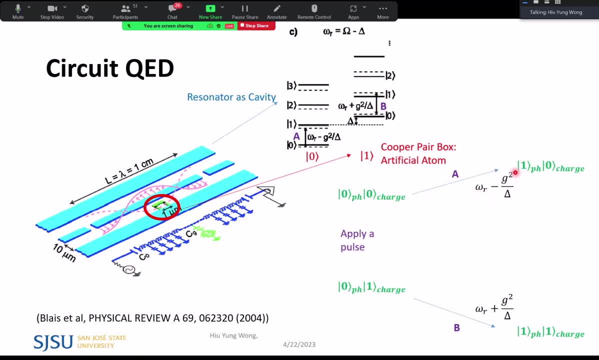 resonator is omega R minus G2 over delta. So if you have zero charge or a zero cooper pair, the energy you need to excite or to include one photon to this resonator is omega R minus G2 over delta. If you have one cooper pair, it is omega R plus G2 over delta. Now no need to memorize this right. 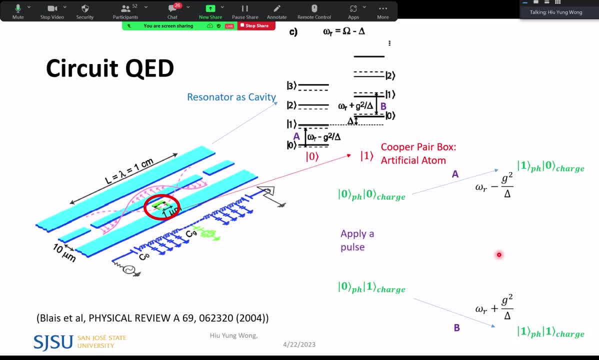 if you feel confusing, But I do want you to memorize that how it works It is that the states of your qubit change the resonant frequency of the cavity. That's it, And because of this the resonant frequency of the cavity is going to change. So I have zero photon and one charge. 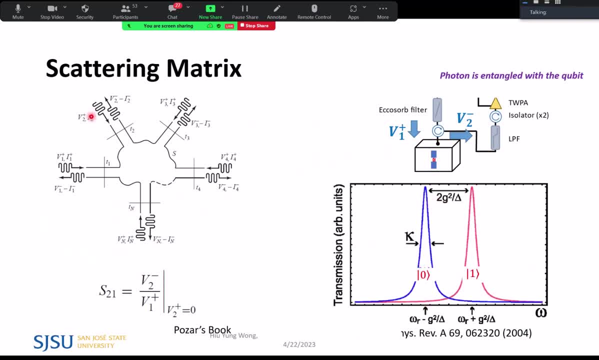 The resonant frequency is changed. Now, if I apply a pulse to it, right, apply a pulse to it, then it's going to have different peak when I measure it, And by doing this I know whether it is in zero and one. So that completes the description of how we measure a qubit in a. 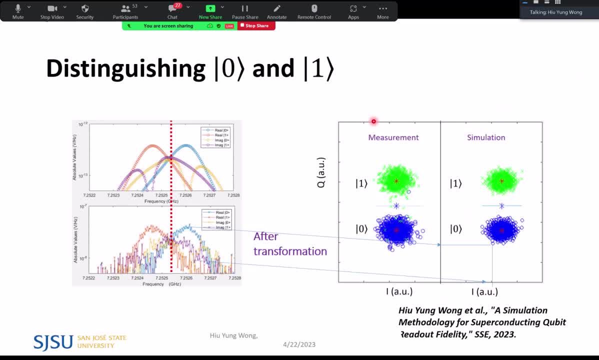 superconducting hardware Here show a simulation in this paper. So what? but it's a good thing to show how it works. We actually measure at a center frequency And because all these microwave puffs, they have real and imaginary parts, because they have a phase, 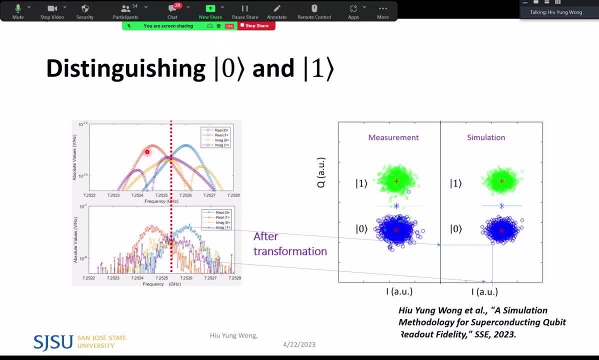 So whether if you are at zero you have a difference. I mean, if your peak frequency shift lower due to zero or shift higher due to one, you have a different real and imaginary frequency. So that completes the description of how we measure a qubit in a superconducting hardware. 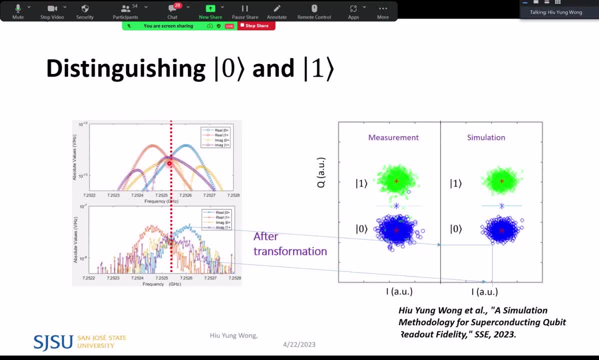 part combination. So when you read it at this frequency right you will have different so-called IQ block. You have the. it show you the in-phase and out-of-phase quadrature, but it's just same as real and imaginary. So because of noise you actually have some distribution. It's not always. 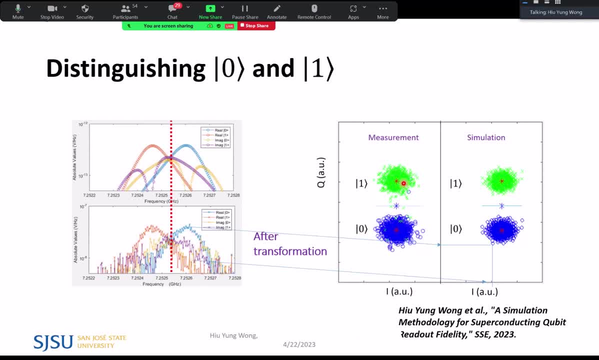 at the center point. So in quantum computing, what you want to do is to set up the device so the separation is large enough, And then I will show you how to do it. So I'm going to show you how to do it. So I'm going to show you how to do it. So I'm going to show you how to do it. So we're going to 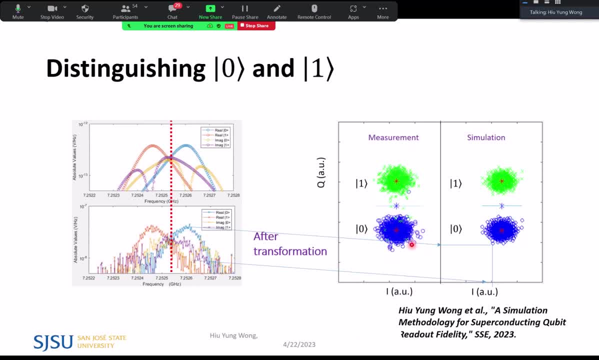 anything above this is one. Anything below this is zero. Again, what is below this? it means the real and imaginary part has this type of combination, And you see that some of the green comes to here because of the noise, And this constitutes the fidelity of the readout. Okay, 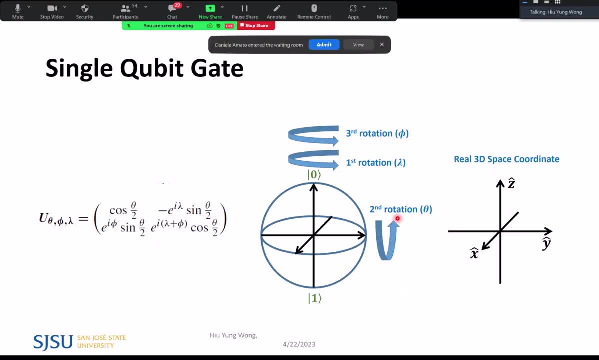 So we're almost done. We know how to do the make the superconducting qubit. We know how to do the readout. Then how do I do a single qubit gate? Here is pretty complicated, No need to understand. But the main point I want you to get is I show you the broad sphere earlier For any. 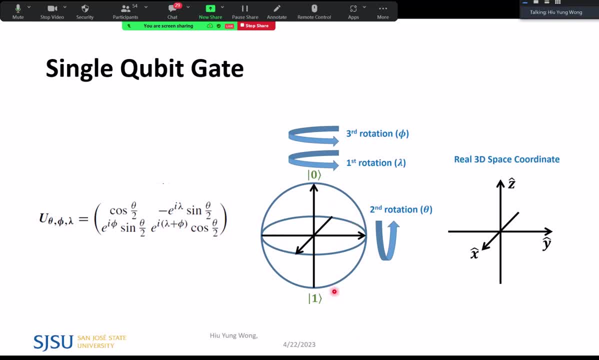 single qubit, the state can be mapped to a broad sphere, So every state is on top of the sphere. So what is a quantum gate? again, It's the rotation of the vector on the broad sphere for a single qubit. Right It is hyperspace. So basically we can use something called Euler rotation to make it. 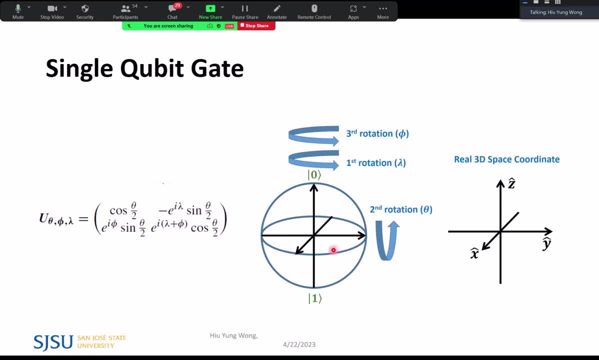 systematic. You can rotate it three times, first above the Z axis and then about the Y axis, and then above the Z axis for different angle. Then it corresponds to this matrix. You can ignore it, But this matrix is useful for us to construct a physical qubit. right Everything I want to. tell you is that a single qubit is already a physical qubit. All right, Let's go back to the thing we talked about before. right, The inner Q was 4, but the inner H was 3.. Just to define the. 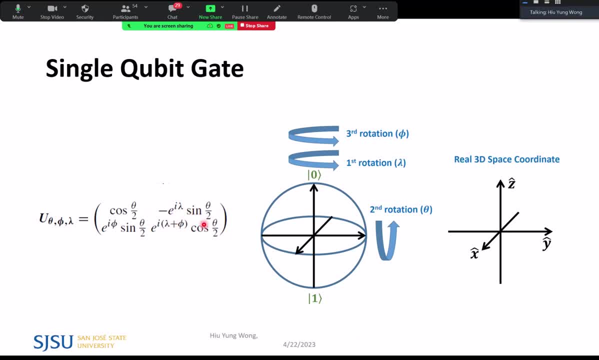 big gates is the rotation of block sphere and we, by getting the correct matrix, then we know the angle we need to rotate. Now I want to emphasize this rotation is not in our 3d space. we just map the hyperspace to our 3d space. but this rotation does have some meaning, correspond to our 3d space. 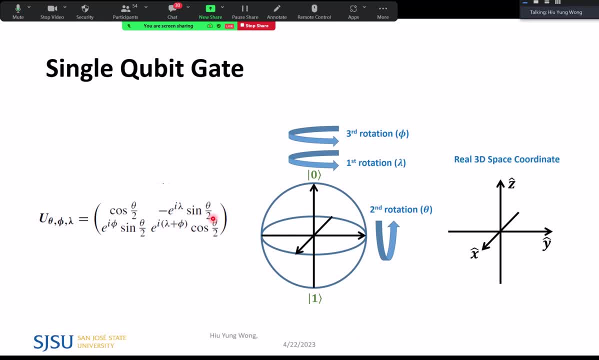 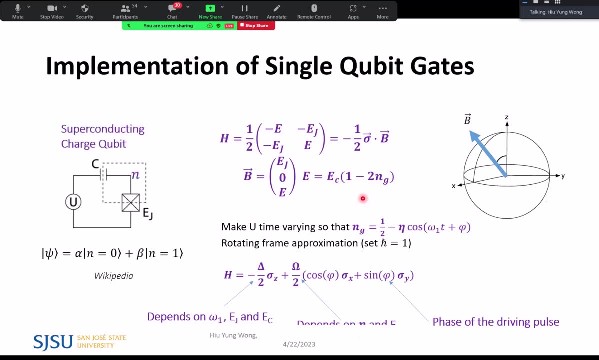 because, for example, in a spin qubit, the 3d space, the z direction, correspond to the magnetic field direction, but however, still we are not rotating in the 3d space. please remember this. So when we implement the superconducting qubit, it is like this: we will apply a gate pulse to here. now we 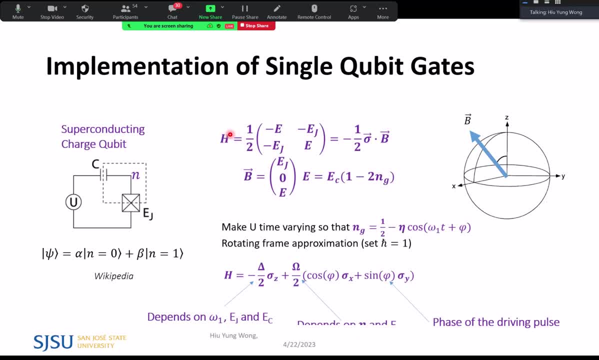 can construct the Hamiltonian which I cannot show here. it's pretty long again. it's in the youtube playlist I showed you earlier quantum computing architecture. we derive from scratch. you will. you will find that no matter is Hamiltonian right. that means the equation, determine how it change can. 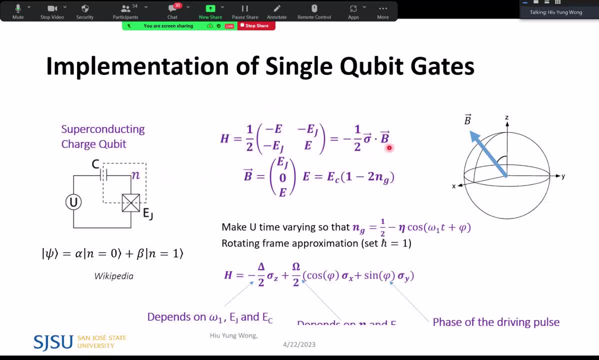 be expressed as this: and this is just like a spin case. it can be modeled as like: I have an effective magnetic field. this is just a mapping. it's not that we have the magnetic field in this system, okay, but why do I want to show you this equation? I want to show a few things. first is that you will 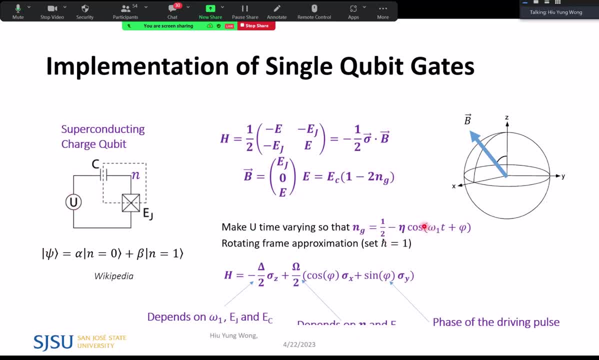 apply the gate pulse with some signal so that you change this ng, which is a part of the e. you see, e is a function of the capacitive energy and also ng, which is the background charge. by changing this voltage I'm going to change the charge here, just capacitive coupling, right? if you are e student, that is easy. 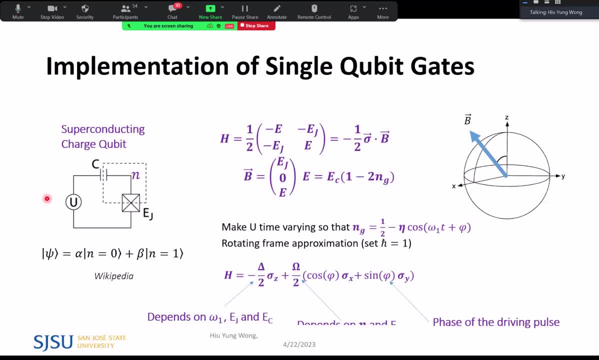 for you to understand capacitive coupling. so if I have a smooth pulse here, I'm going to change the e to some small signal. all right, eventually you find that this Hamiltonian is equal to this. the only thing I want to show you is that this is mapped to a spin qubit, so in a spin qubit, I think. 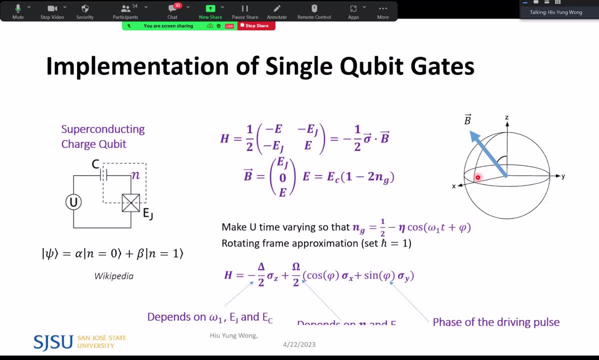 you all kind of understand: a spin on the magnetic field, it will precise, it will rotate about the magnetic field, right? i map this to here. it is the same. it's going to precise, and that is the same, and rotate about this block sphere so that i can, uh, get any arbitrary one cubic quantum state. 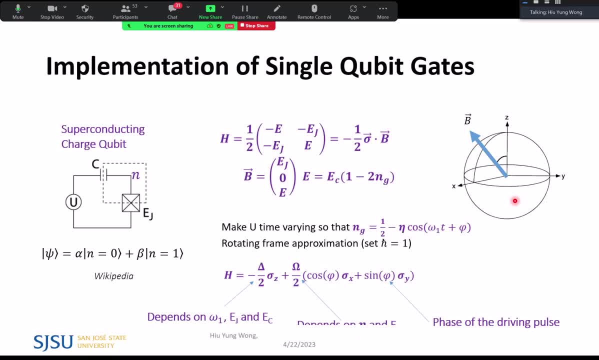 and i can move that quantum gate and i can move it to any place, right? but i want to show you. you see, delta depends on josephson's energy, capacitive energy that we mentioned earlier. this omega depends on eta, which depends on the gain voltage you apply. it also depends on the 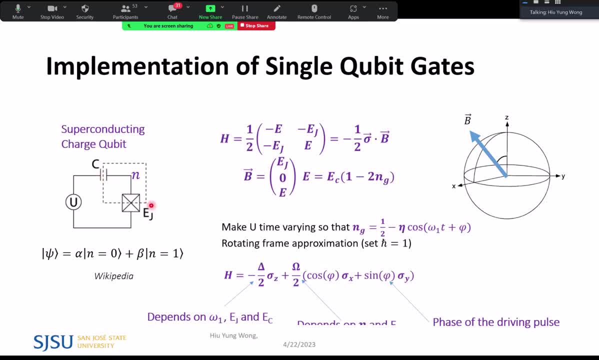 phase, which is very important. it depends on the phase of your driving pulse. so you see that quantum computing is very, uh, delicate. it has a, you know, very good control on the pulse that you are sending to the qubit, including its phase, not just its noise from other sources. 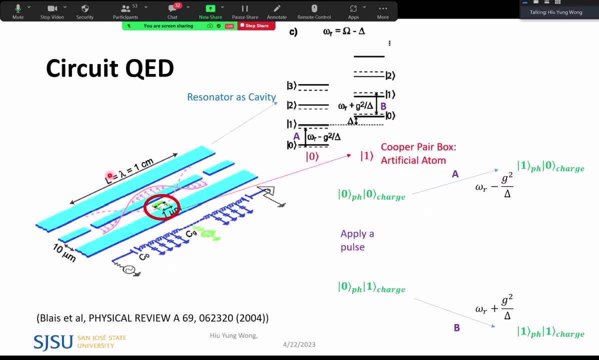 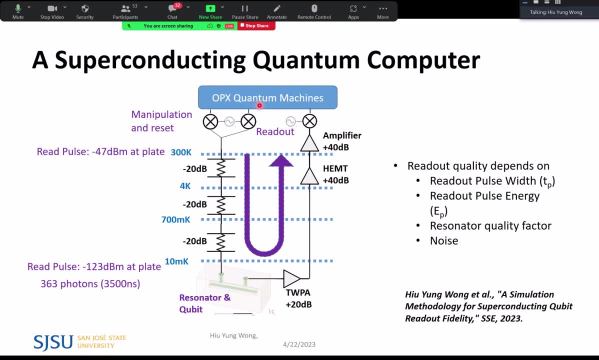 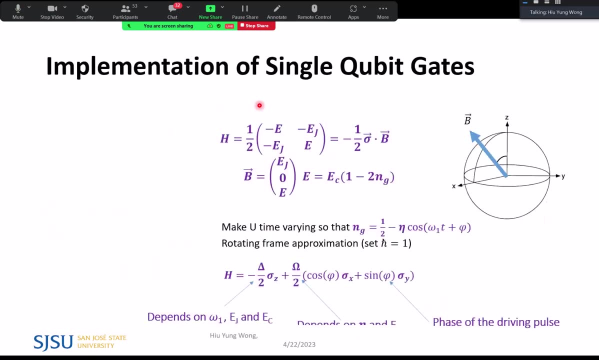 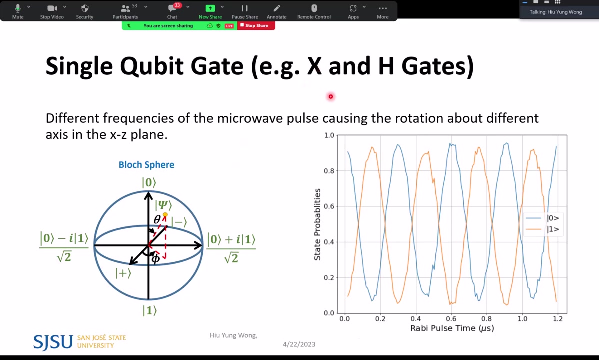 its frequency right and that's why earlier i showed you that people like quantum machines. they just sold this system for a lot of money because they have a lot of fpga and algorithm and interface to make this easy. okay, so there is single qubit gate, for example. here we can apply the x and hadamard gate. 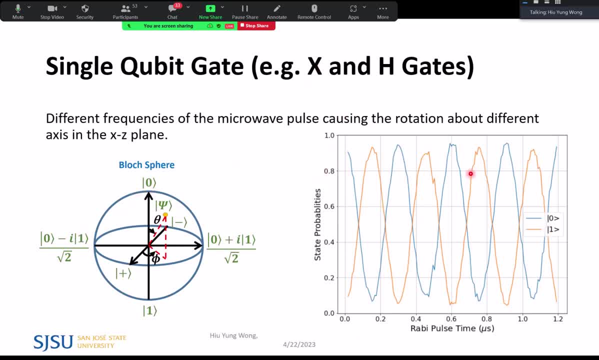 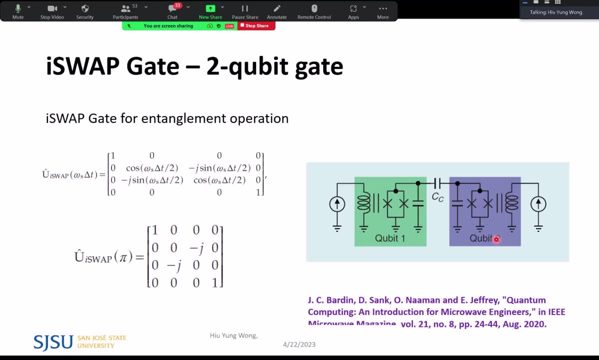 and then we can let it oscillate from zero to one, zero to one right. finally, i will talk about the two qubit gates. uh, we won't. i cannot go too too deep, but basically for quantum computing we talked about c-node gate, right, but it's not just c-node gate that is. 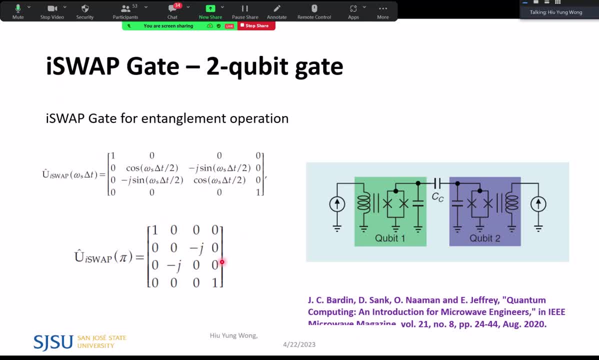 useful. you can also use i-swap gate. this is the i-swap gate and in for this gate it has. it is also an entanglement gate. so if you you can transform the c-node gate or other operation to using i-swap gate for different uh quantum computing architecture, you will see people use. 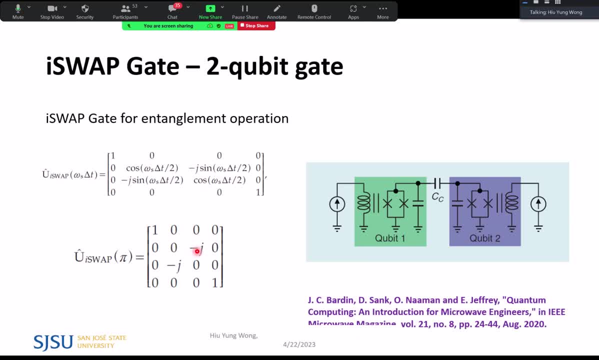 different entanglement gates because of the physics. we are using the physics to implement it. for example, in a spin cubic case, they actually use the control phase shift gate instead of i-swap gate or instead of c-node gate, because it's easier to implement due to physics. in this case i have two qubits, of course, because it's two qubit gate. 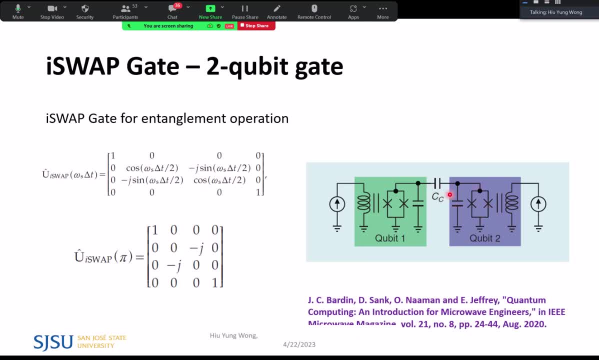 and what they're doing is rely on this coupling of this capacitor. so a hand waving. understanding given by this paper is that you can be zero zero one one. right again, what is zero zero one one? it's related to the energy. they have different energy, so if they are both at zero zero one one, just like a classical circuit, they are not. 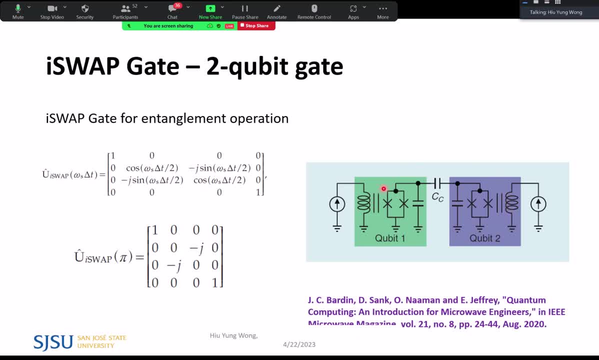 going to exchange energy, so the state is not going to oscillate between them. but if one of them is zero, one is one, then they will start oscillating right. and this is. this can be seen from this matrix. the first one is correspond to zero, zero. the last is: 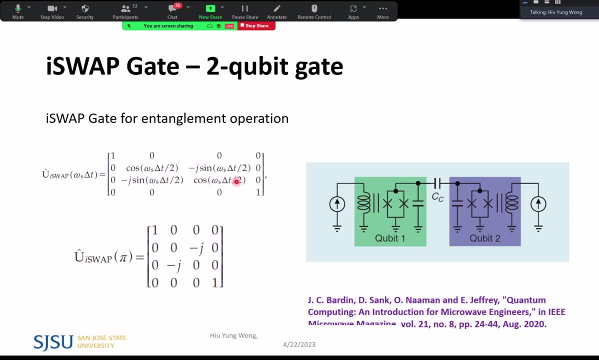 one one right if you understand the matrix well, but otherwise this is okay. you with this type of oscillation, you just do the time correctly. you want to turn on them so that you change their coupling and also energy difference. it's not shown here full and other circuit. 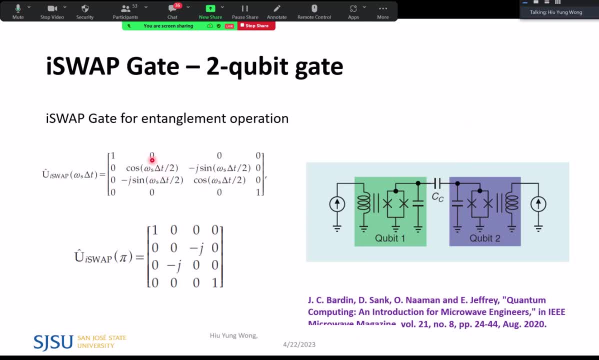 this oscillation and then you do the right timing, you can make this to zero. when this is go pi over two, this is zero and this is equal to one right. so again, a very precise control is important and i guess you understand why there's so much error: not just the noise, but also the control. 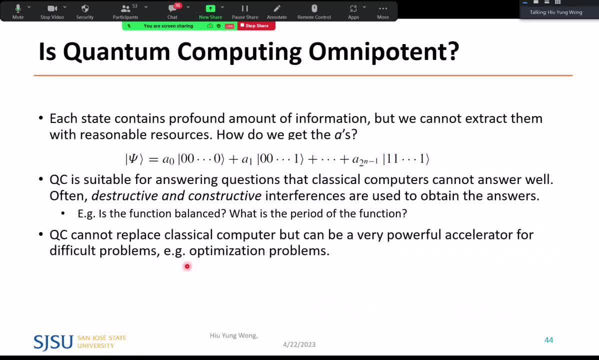 okay, so that's almost the last line, right? so i try to cover from the basic algorithm all the way to the hardware. i hope you have some idea of what quantum computing is about. i want to say you see that we are, with 100 qp, 300 qb, i get a lot of information. 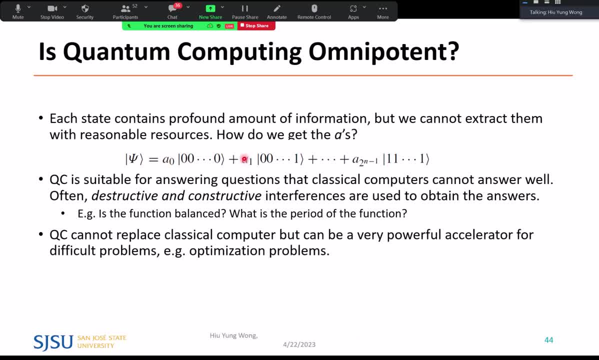 but unfortunately it's in the qubit. i cannot get a zero all the way to a to the power and minus one. then what should we do? we need to use constructive and destructive interference or some smart algorithm that use this interference so that it tells us the answer that we want, for example in: